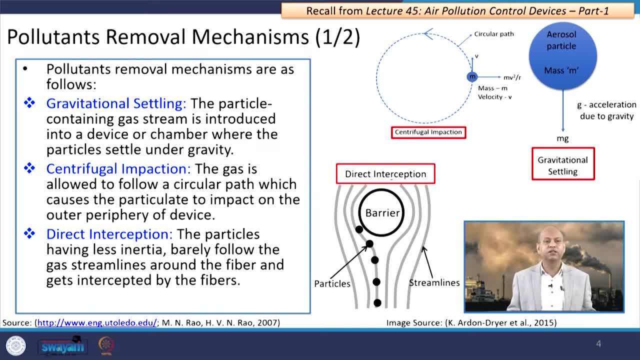 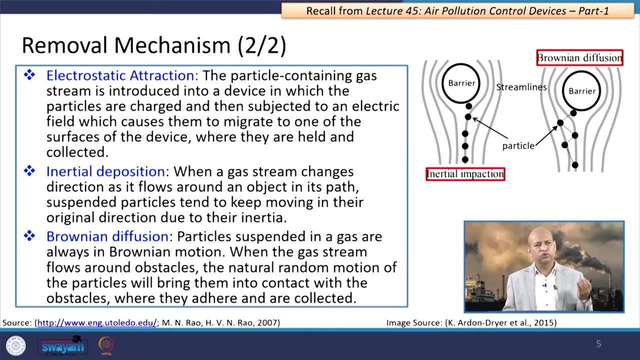 Then direct interception can also be there, like the particles having less inertia, like barely follow the gas streamlines around the fiber and gets into intercepted by the fibers itself. Those kind of interception occurs. Electrostatic attraction is also one way of controlling these air pollutants or collecting these air pollutants of particulate nature. 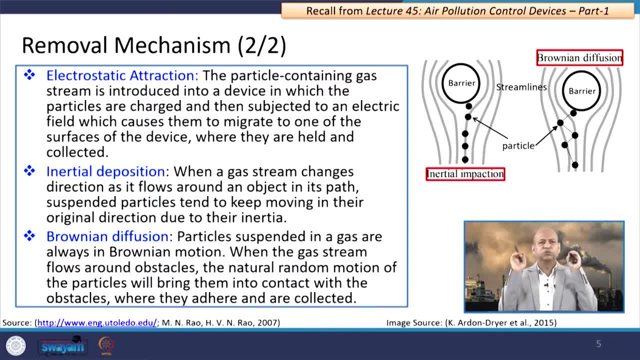 The particles containing gas stream is introduced into a device in which the particles are charged and then they are subjected to an electric field which is causing them to migrate from one of the surface of the device to another surface where the opposite charges are there. Then they lose. 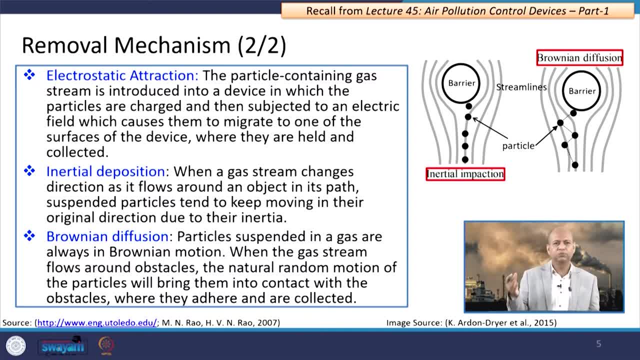 the charge and again slide down and get collected into the bottom hopper. Then there is one mechanism like inertial deposition, in which gas stream changes direction as it goes down. So this is one way of controlling the air pollutants. So this is one way of controlling. 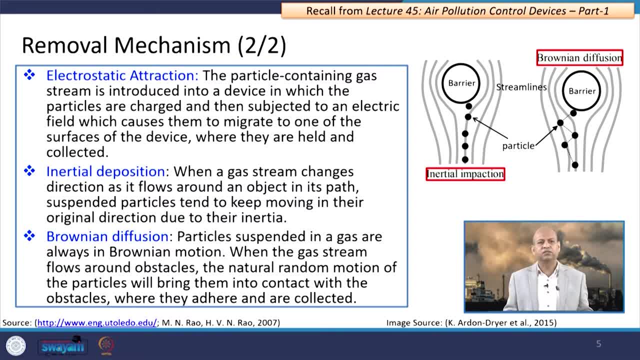 the air pollutants. So this is one way of controlling the air pollutants. So this is one way. it flows around an object in the path and suspended particles tend to keep moving in the same direction and they strike with the inertia, strike to that particular object and again, 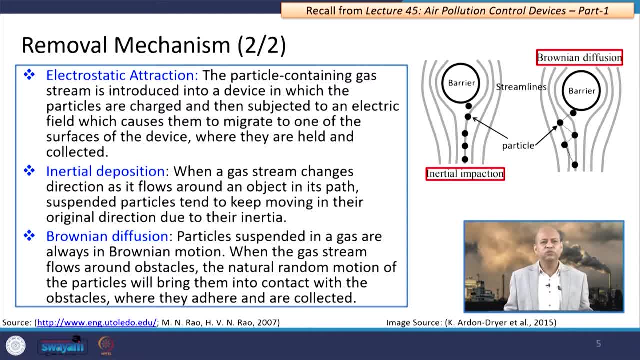 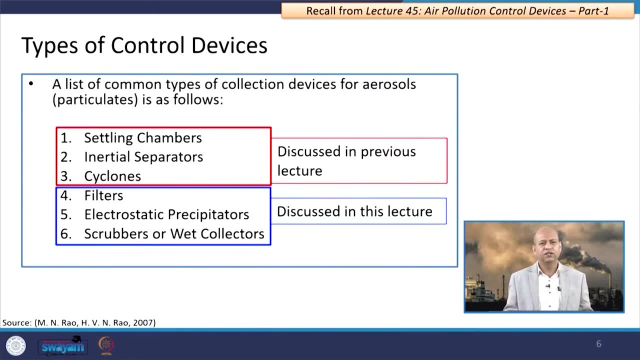 lose the velocity. Then there is Brownian diffusion, also like particles they are suspended in the gas and they always in Brownian motion. they go from one direction to another and in that movement they again get impacted on the the surface and then get reduced to the like velocity, get reduced to the 0 and then they 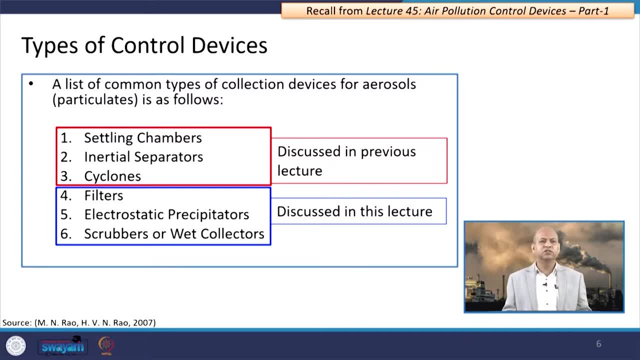 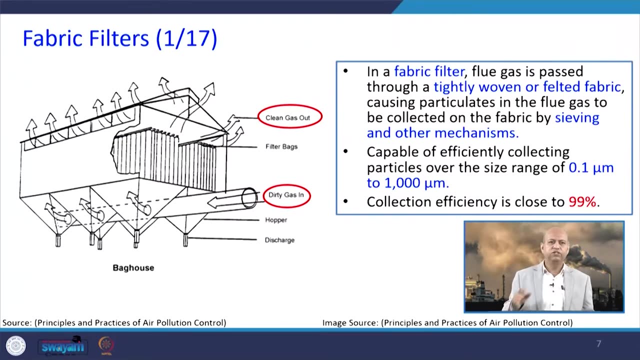 slide down. So in that way we have discussed three devices like settling chambers or inertial separators and cyclones. in the last lecture Today we will cover filters, electrostatic precipitators and scrubbers or wet collectors. So when we go to the fabric, filters basically, 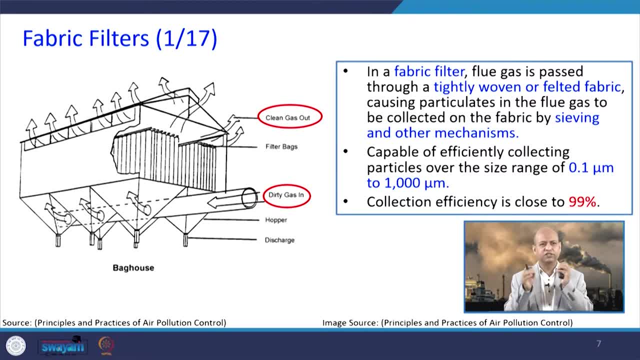 in fabric filter. this flue gas, which is containing particulate matter, is passed through a tightly woven or like cloth or fabric bag or something like that. that causes particles in the flue gas to galactate down the fabric by like sieving kind of thing, because it pass through the 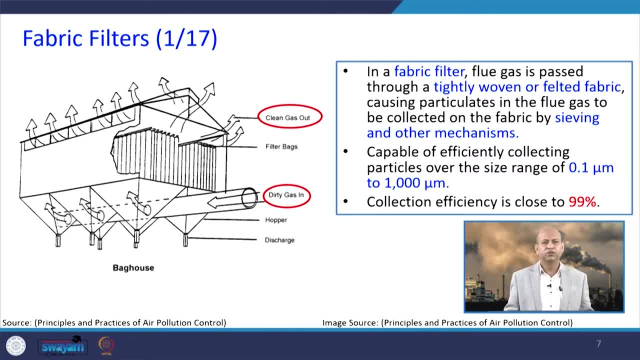 pores and then it get attached to those surfaces and these are capable of efficiently collecting these particles. So very good range is there for fabric filters. They are very good devices when, in fact, to control or to capture very small particles and even large particles. So 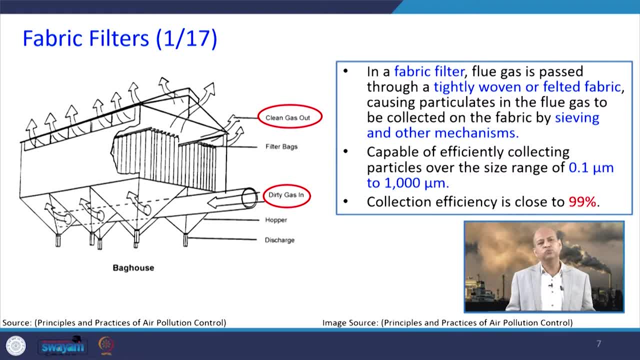 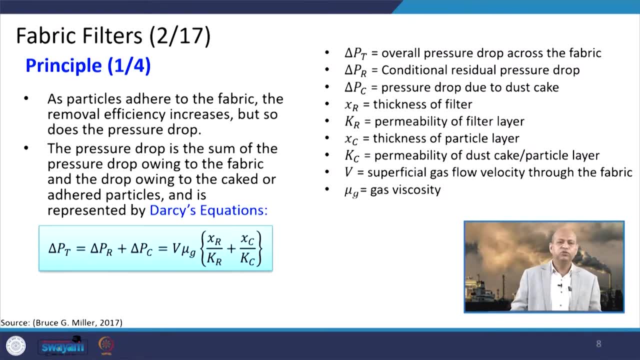 that way it is very good. and then the collection efficiency is also very high. like 99 percent of the particles can get collected by these fabric filters. Now if we talk about the principle- how does fabric filters operate- then basically we should know about the concept of like overall pressure drop. when something is coming, then they pass through. 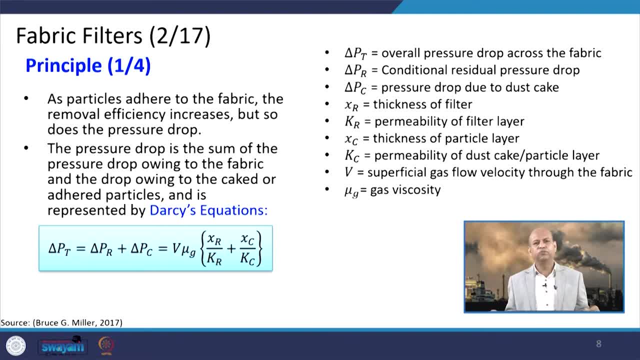 some inertia or some kind of obstacle, then they loses this force or pressure. So overall pressure drop is causing in the across the fabric filter that we should know. then this conditional residual pressure drop, delta PR, that is also to be known. Then pressure drop due to dust cake- cake means the dust cake. 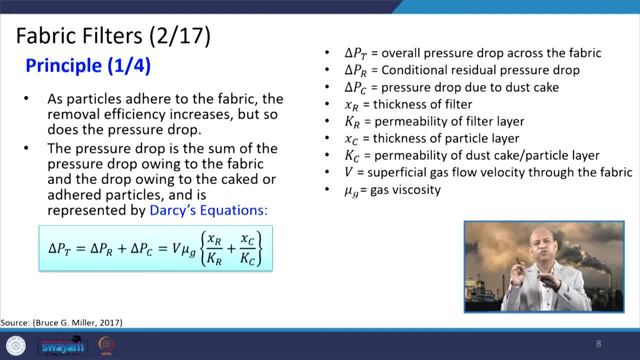 It means the dust particles which will get collected on the surface, So ultimately they will form some layer, or we call it cake, So that because of that also pressure drop will be there. Now, thickness of the filter that fabric back house filter, and then permeability of the filter layer. 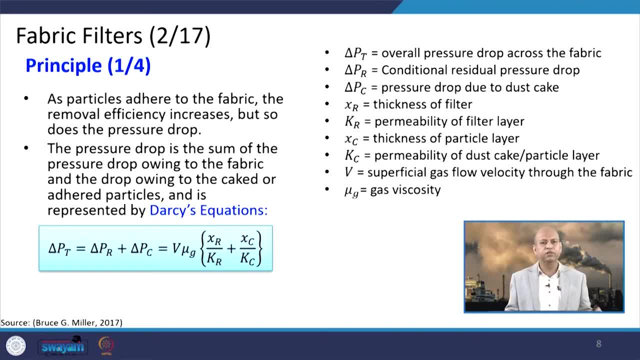 thickness of particle layer which will deposit over the period of time, and permeability of that dust cake, or the particle layer that should be known. and superficial gas velocity through the fabric filter. when gas is passing through with certain pressure drop, So it will get collected. 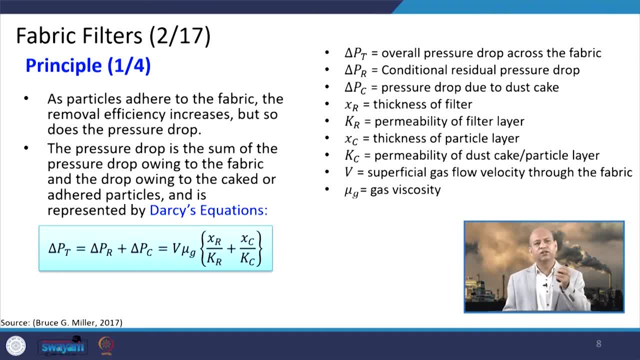 through with certain velocity and gas velocity, this gas viscosity, mu g, that should also be known in addition to the gas velocity. So those things, these all parameters can be put in this equation and we can get this delta pt, that is, the overall pressure drop, by using these particular values. 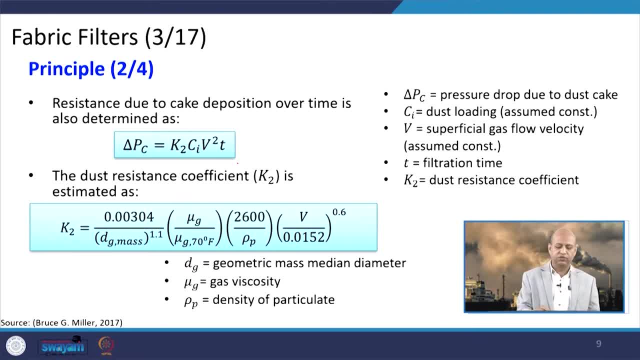 Well, when we talk about, like, resistance due to cake deposition, that can be calculated further with this empirical relationship, and where k2 is basically dust resistance coefficient, that is also calculated by this empirical relationship, which has density of the particulate gas, viscosity, then dg, is there this geometric mass median diameter. 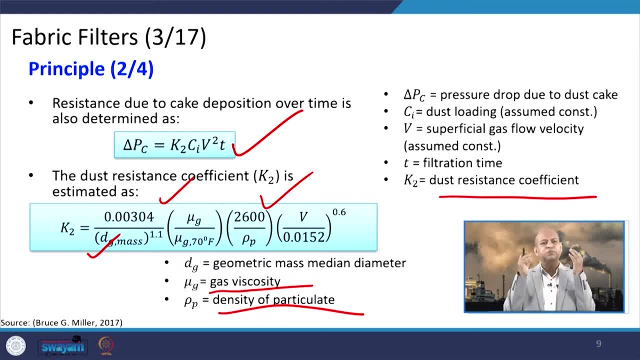 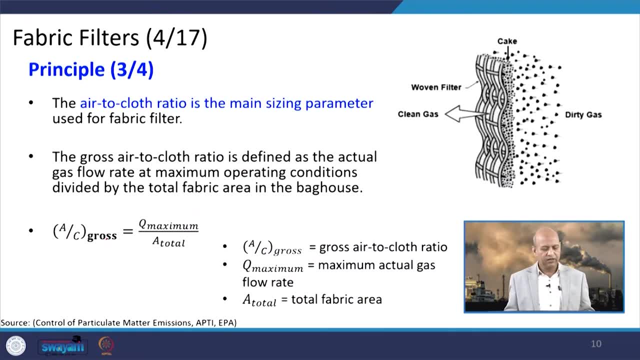 because particles are of different sizes. So we calculate the mean or median diameter of those particles that is to be used for this calculation purpose. Then, when we talk about like air to cloth ratio, that is also very important governing factor for efficiency of collection of particles through fabric filters. 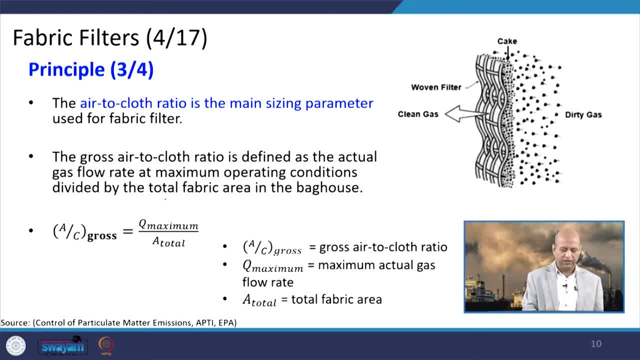 So this is basically you can call like. this is ratio, which is defined as the actual gas flow rate at the maximum operating conditions divided by the total fabric area in the bag house. So that is the air cloth ratio which is a parameter, And this air cloth ratio, the gross, is Q maximum divided by A total. 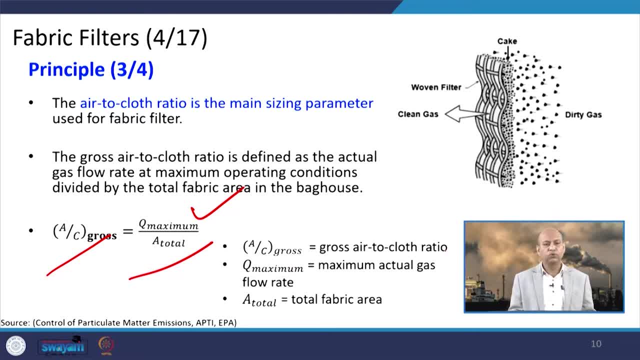 So A, this gross of the air to cloth ratio is calculated by this particular relationship, where Q maximum is maximum actual gas flow rate and the actual gas flow rate of the maximum value, because it may fluctuate. So the maximum value we will take and the A total fabric area, the complete fabric area. 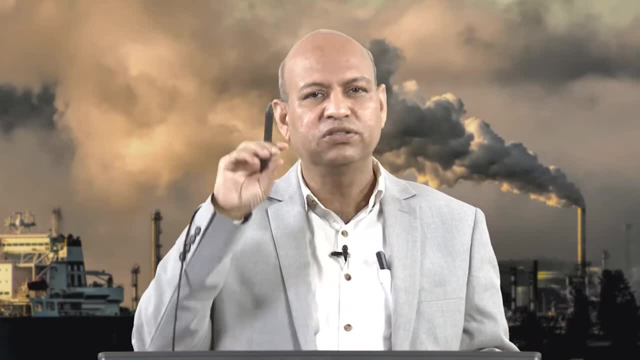 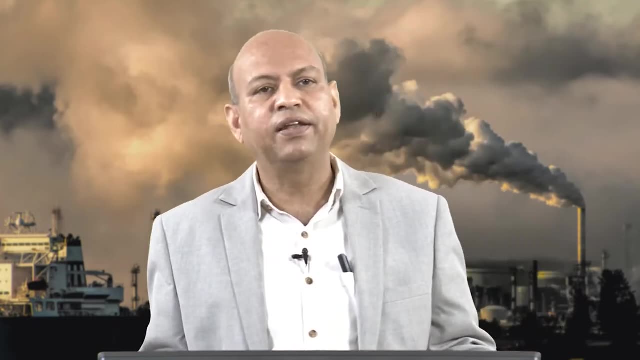 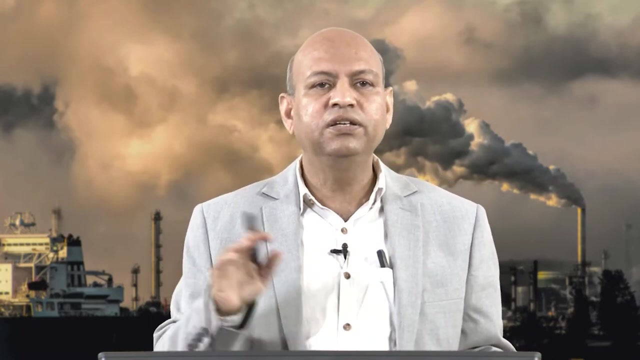 through which this gas will pass. So that area has to be taken means including the pores. Including the pores? Well then, there is another concept of the net air to cloth ratio, and this is basically defined like it is: the multi compartment fabric filters, where one or more of the compartment 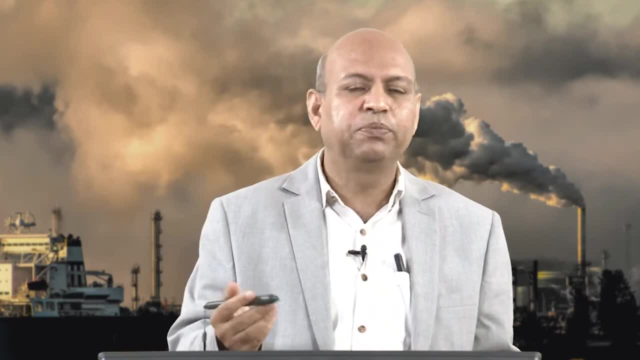 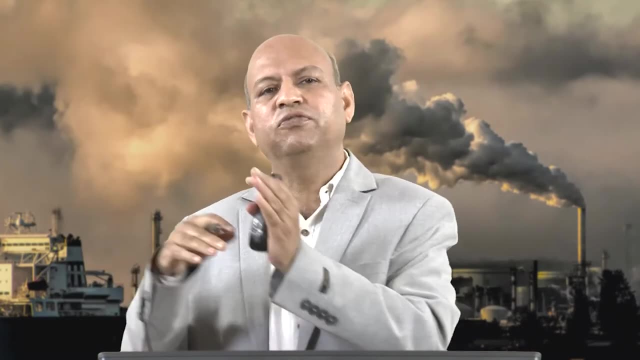 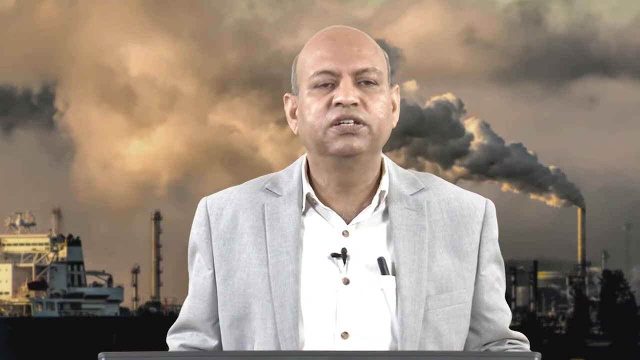 is isolated from the gas flow due to, like, cleaning purpose or maintenance purpose. So there may be multi filters or bags- Yes, Bag filters, So one can be for maintenance purpose, others may be in operation. So in that case, this net A, oblique C air cloth ratio in terms of net. 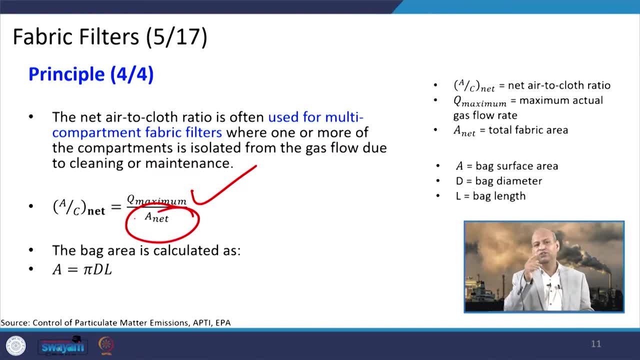 So that is Q maximum divided by A net Earlier we used A total total area. now this is the net area which is in operation and in A total basically we are. we use all kind of these cloth area, So in this bag area is calculated. 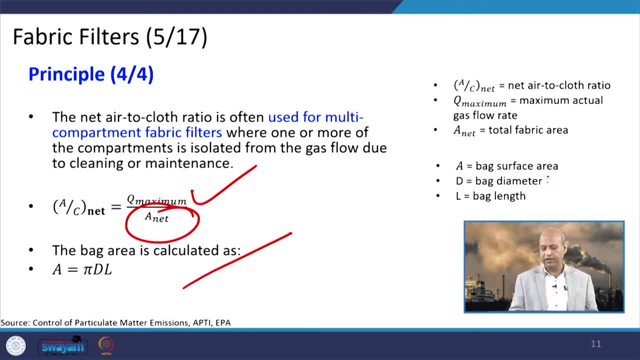 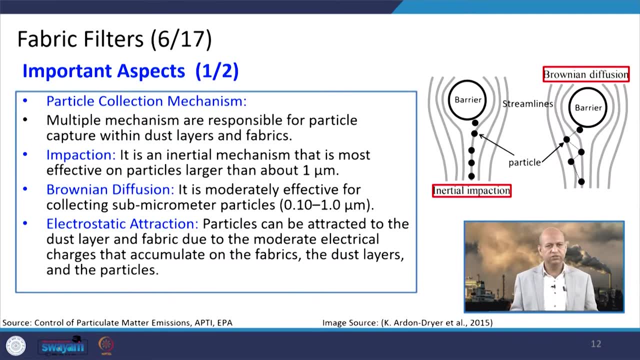 So bag area is calculated by pi DL, where D is the bag diameter and L is the bag length and A is the bag surface area. So this is the relationship which is used for calculation of this air to cloth ratio of the net, not the total total was earlier one. 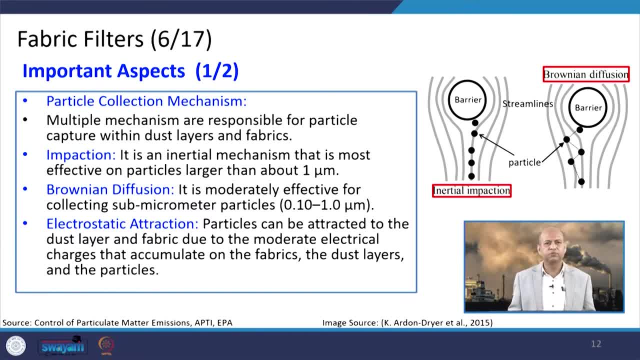 Now there are different important aspects in filter. this fabric filter operation, like particle collection mechanism, is important in the sense that these multiple mechanism are responsible for particle collection. Yes, So this is the material capture, with the dust layers and fabrics like impaction brownian. 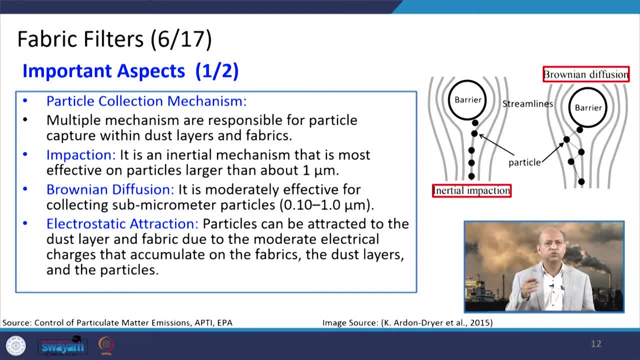 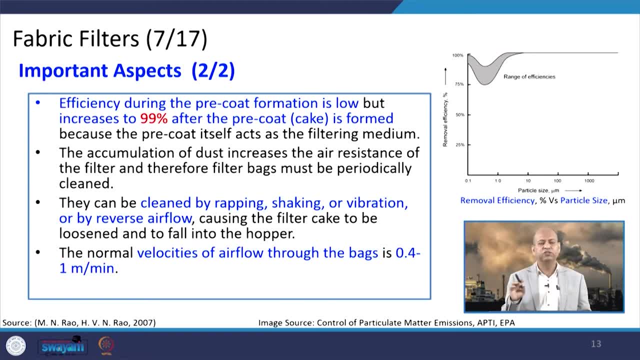 diffusion, electrostatic attraction. So those things are important aspects basically. And then if we talk about the efficiency during this pre coat formation, that is, before cake formation of the particle layer formation on the bag, So then it is less efficiency. but after this layer is formed then efficiency increases. 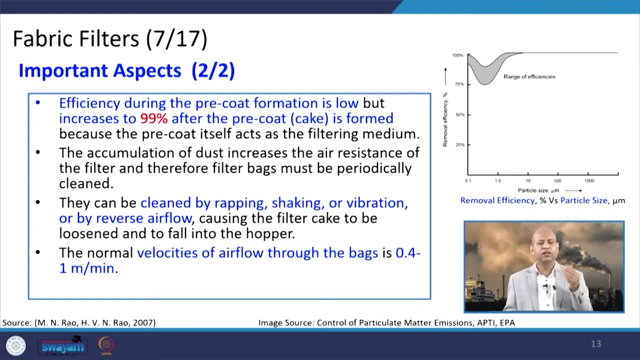 because then more it is like pore is less In size or less area is available to go through the empty area. So the efficiency increases. basically, when this pre coat in comparison to the pre coat there is, this dust increases and that air resistance increases because of less pore. 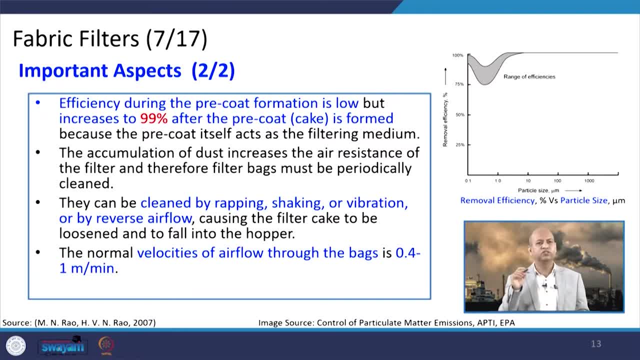 size. So the cake formation is also important in this case. basically, And this normal velocities of air flow through bag is 0.4 to 1 meter per minute. So that kind of velocity. So velocity has to be there, otherwise you can see like particle size and this removal. 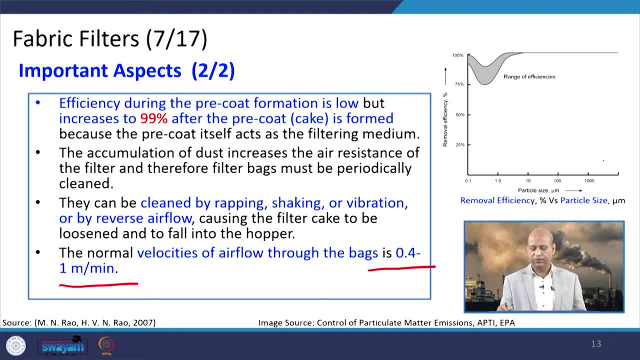 efficiency. that can vary basically for different sizes, but you can see this kind of drop is there for some particle size which can be again overcome when cake formation. is there Those particles, this like 0.1 to 10, so their efficiency is less initial stages but after. 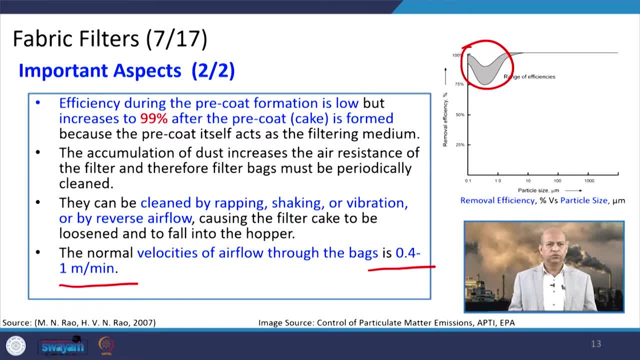 cake formation, the removal can be better. So in contrast, So in continuation to the important aspects, we also consider, like pre coat formation, Before this cake formation is there, efficiency is less, especially in the range of these particles, 0.1 to 10 micrometer. when this coat formation or cake formation is there. 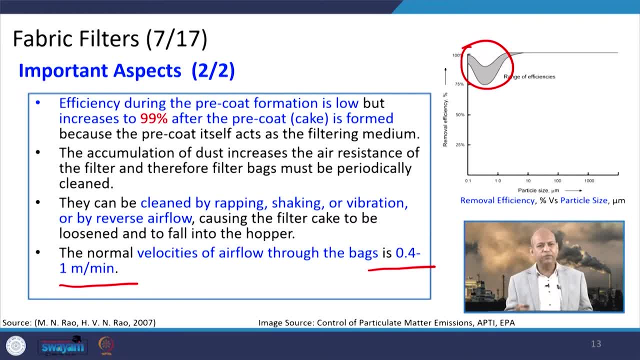 then resistance is more for passing the air and then the efficiency again increases and this like, for example, it is around 75, then it becomes like maybe 85 or 90 or something like that. So that way the efficiency increases after this cake formation and the normal velocities. 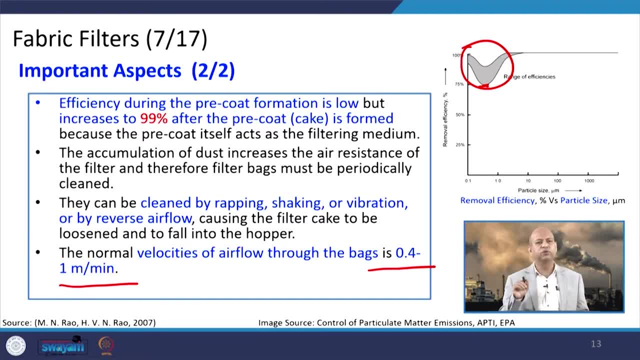 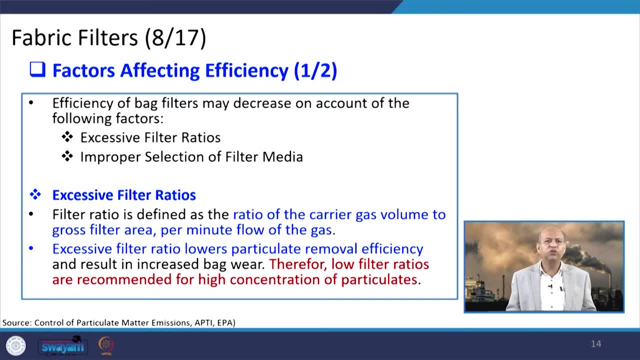 of the air flow through these bags has to be like 0.4 to 1 meter per minute, So that way we can collect a lot of particulate matter with good efficiency. Then if we talk about like efficiency of bag filters, how they decrease or increase, so 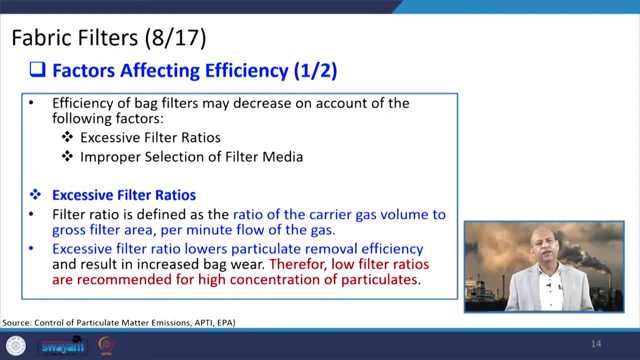 they may decrease on account of following factors like excessive filter ratios or improper selection of the filter media. So those could be Could be the reason basically When we talk about excessive filter ratios. basically, this filter ratio is defined like carrier gas volume to the gross filter area per minute flow of the gas. and this excessive 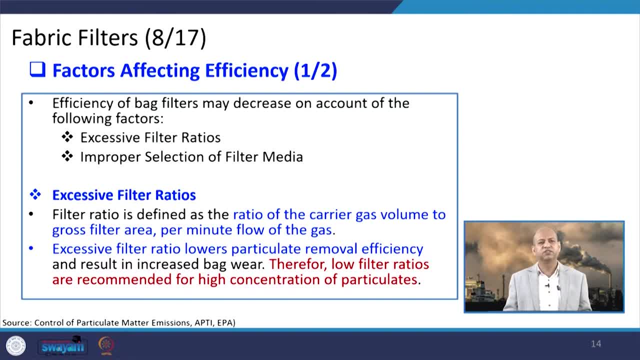 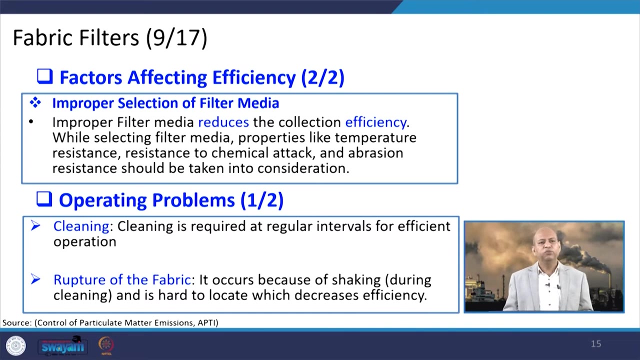 filter ratio lowers particulate removal efficiency and result in increasing the bag wear and tear, So that way life of the bag also is reduced. therefore low filter ratios are recommended for high concentration of particulate matter to be removed. Then we talk about like improper selection of filter media, so improper filter media. 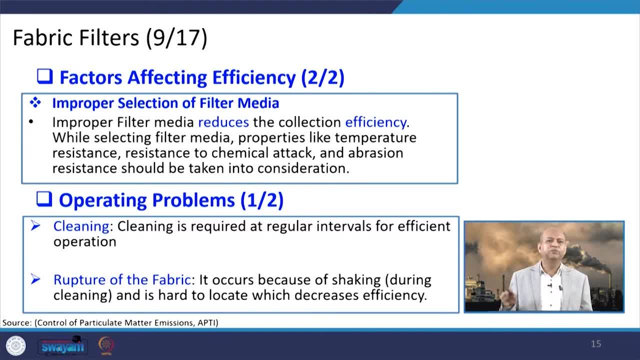 can reduce the collection efficiency. also, While selecting filter media, properties like temperature resistance means because the gas, these emissions could be of different temperature, basically. so what is the range, which range of the temperature this filter media can afford? So that has to be considered. 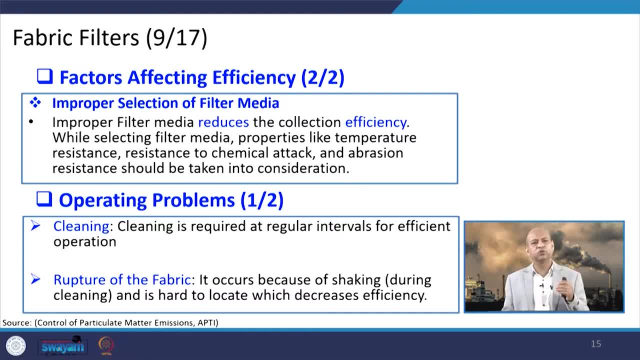 So that has to be taken into account. Then resistance to chemical attacks, because some gases may be of acidic nature, like SO2, etcetera, may be there. So if dew point is achieved, then the sulfuric acid formation may be there because of moisture. 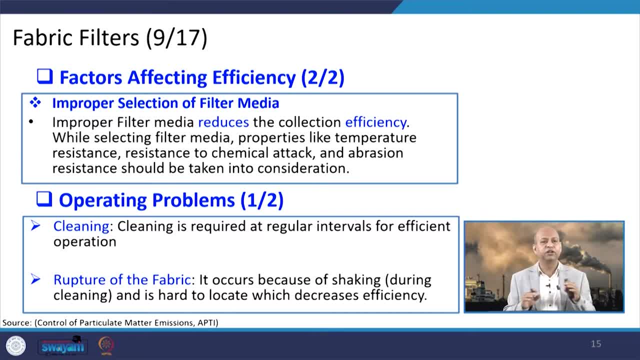 etcetera, and this can attack the filter media. if it is not resistant to chemical attacks, Then abrasion resistance or all these kind of things should be taken into consideration. basically, When we talk about operating problems means operational problems, Then cleaning, rupture of the fabric. so cleaning is required because otherwise when 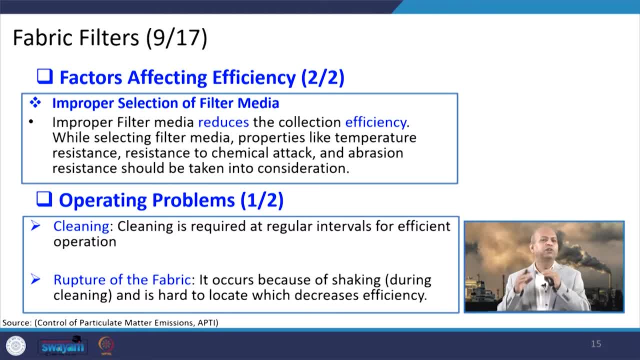 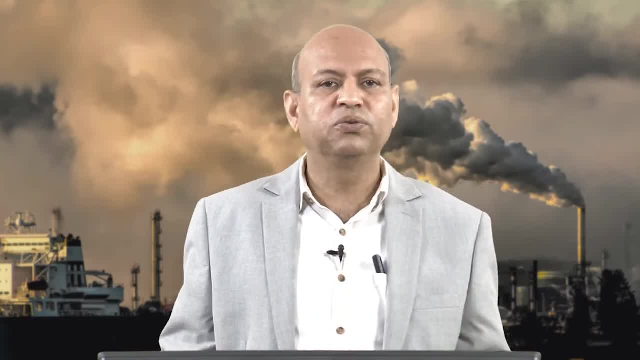 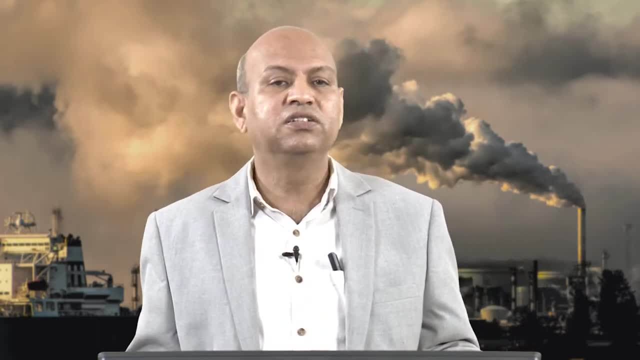 these pores are packed, then pressure drop increases very high and efficiency decreases. So regular cleaning has to be there. Then rupture of fabric can be there because of shaking during the cleaning process. So it is very difficult to locate that rupture and it can decrease the efficiency very significantly. 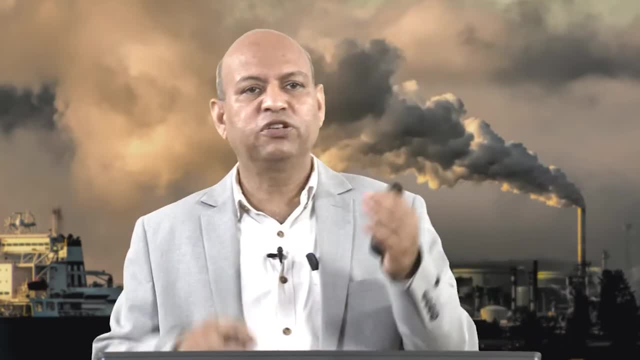 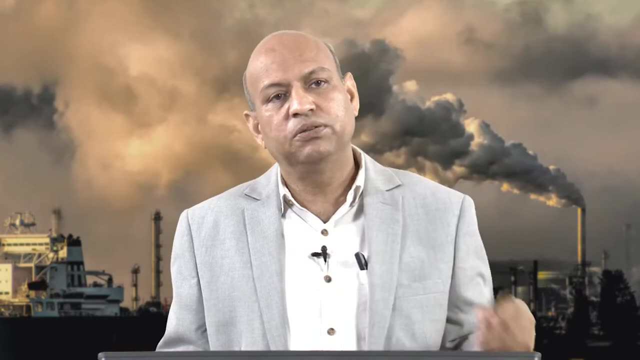 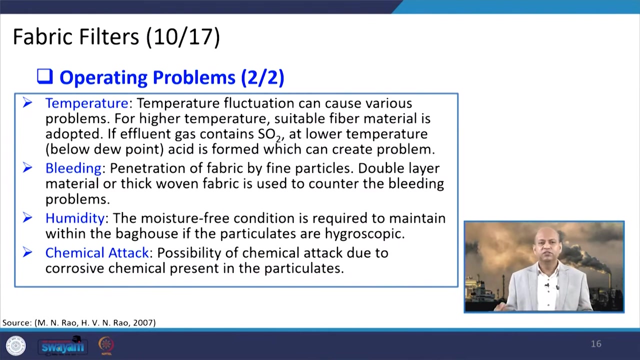 Then temperature also, Like if temperature fluctuation is there and very high temperature occurs, maybe fire can also can be caught by the filter media if it is not very high. temperature resistant Bleeding, like penetration of fabric by some fine particles. Double layer material or thick woven fabric is used to counter these bleeding problems. 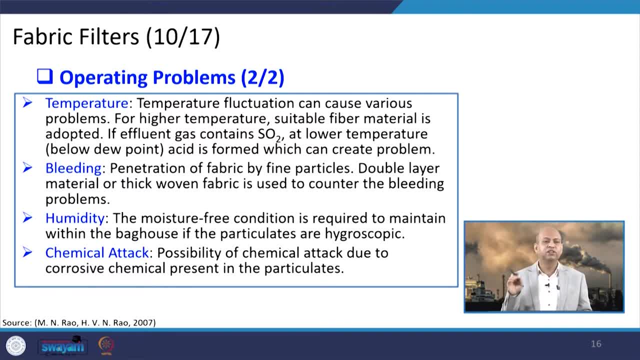 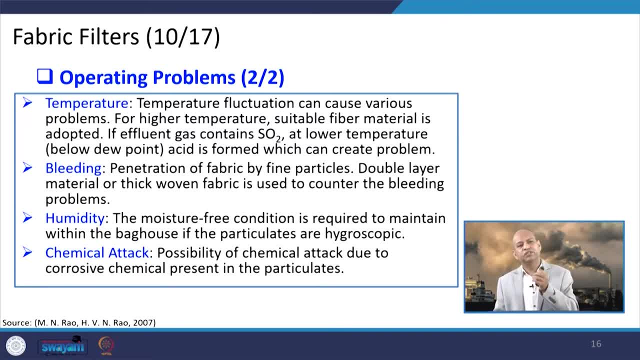 So this is very important. So this is very important. Otherwise, particulate matters of hygroscopic nature, they will catch the moisture and they will deposit to the pores. It will be difficult to take them out. and the efficiency or the removal efficiency and 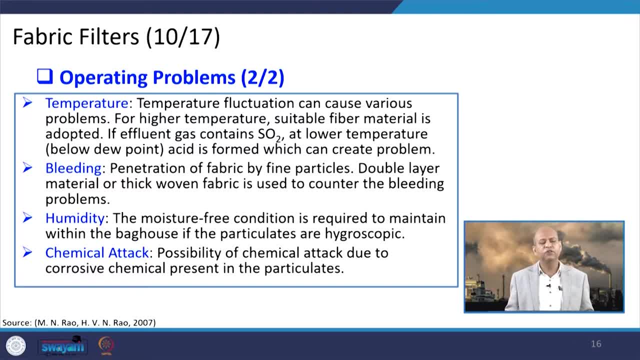 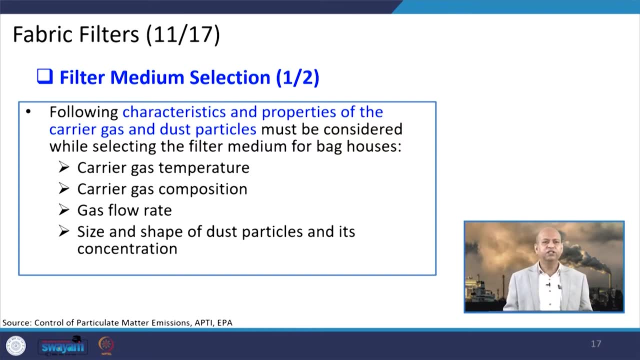 this pressure drop will increase and efficiency will decrease. Chemical attack- as I said, possibility of chemical attack due to corrosive chemical present in the particulate matter and gas can be there. Then if we talk about, like Different characteristics, which are important, different properties of the filter media, which 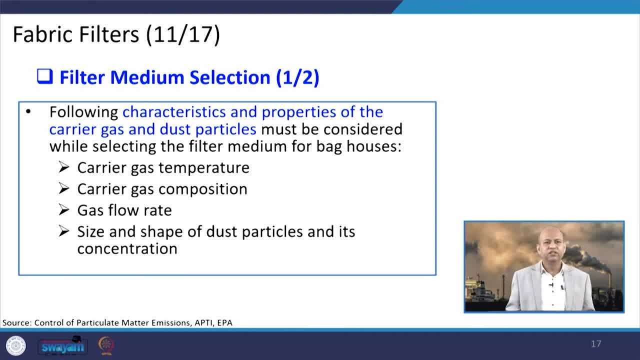 are important for this bag: house filter or fabric filters. These are like carrier gas, temperature, carrier gas composition of SO2, etc. If there, then we have to take care. those kind of filter media we have to select which can resist the chemical attacks, Gas flow rate, size and shape of the dust particles and its concentration, because accordingly, 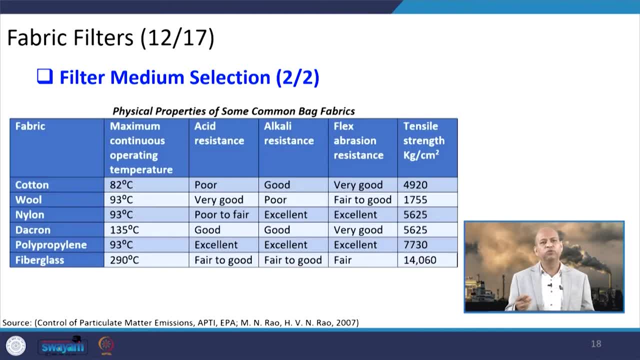 you know, the pore size will vary, Efficiency, Efficiency of removal vary, All these things will vary. So if we see this table, you know this gives the physical properties of some common bag house fabrics like cotton. Cotton is there. then the maximum continuous operating temperature could be 82 degree Celsius. 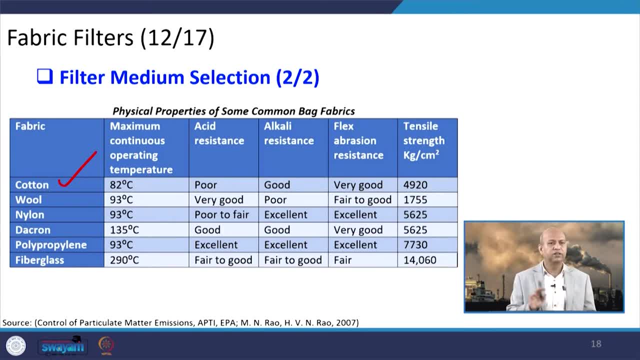 Beyond that, you know fire will be there. So we cannot increase the temperature beyond 80 or 82 degree. Acid resistance is poor for cotton. They can attacked by resist acidic component of the gases and their life will be very less. Average. abrasion resistance is good for the cloth, this cotton, and then flex abrasion resistance. 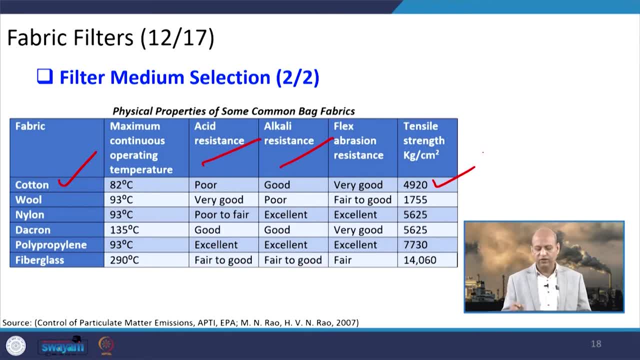 is very good in that sense and tensile strength is around, you know, 4900 kilogram per square centimeter. This is better than the wool. but wools temperature resistance is better: 10 degree Celsius It is. wool is good for acidic resistance. then it is fair to good for these abrasion resistance. 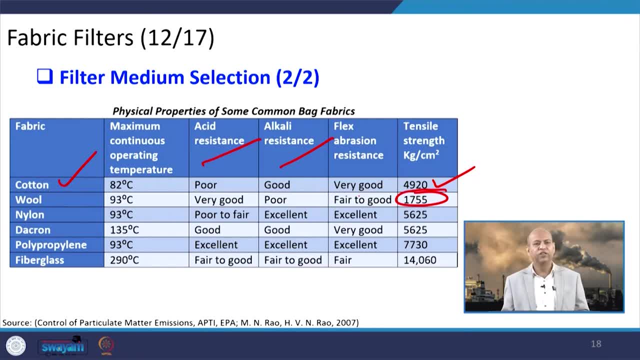 but the tensile strength is like only 1750.. Much less than the cotton. one Nylon has, you know, similar properties as wool when temperature is taken into consideration. but acid resistance is, you know, not so good in comparison to the wool. or then alkaline. 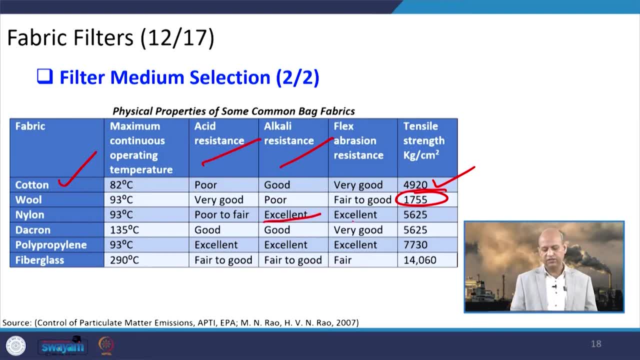 alkali resistance is excellent and this abrasion resistance is also very nice and this tensile strength is better than the wool and means even better than the cotton. you can say Then other materials are there. the best one is, you know, you can see here fiberglass, which 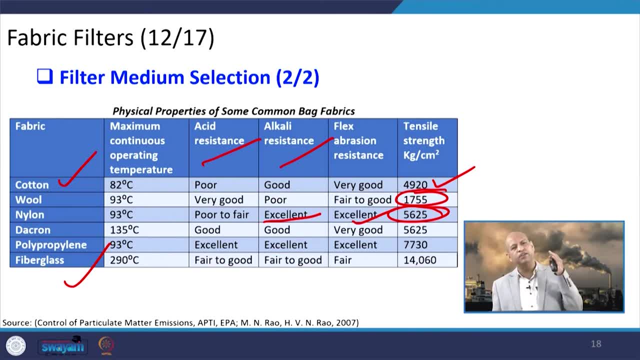 is having very high temperature resistance, like up to 290 degree Celsius it can resist, and but acid resistance fair to good. basically, it is not excellent like polypropylene, So it is fair to good. Similarly, alkali resistance is also fair to good and flex abrasion resistance is fair. 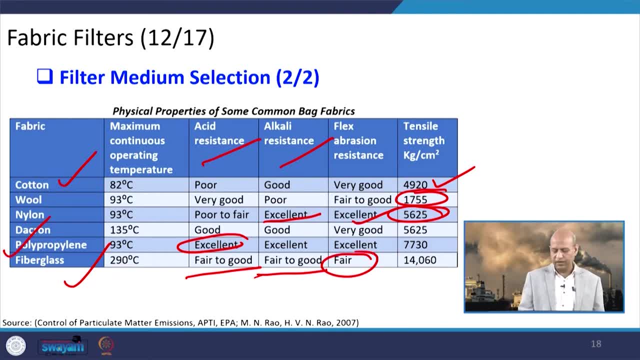 not excellent. This polypropylene has excellent properties. It is very good. It is very good. It has excellent properties for abrasion and resistance to acidic and alkaline components and tensile strength is maximum for this fiberglass. but second best is this polypropylene material. 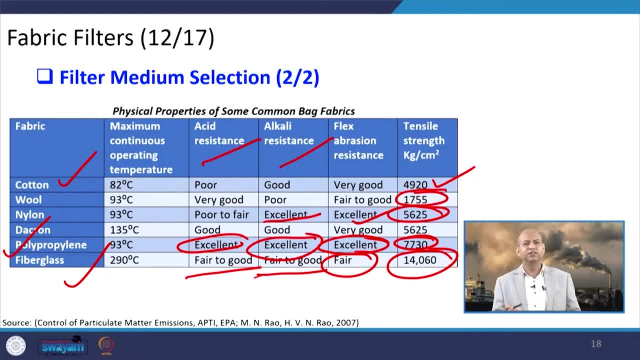 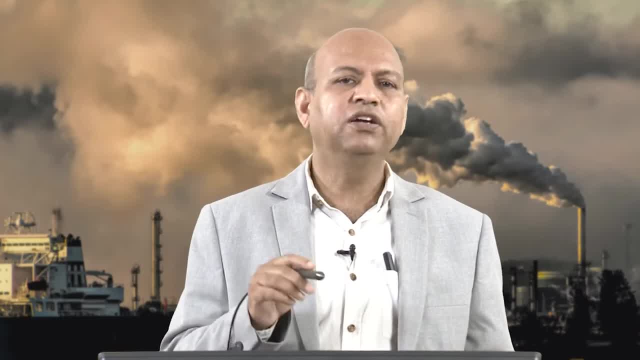 So means, depending upon which industry is there, what kind of gas it is coming, what is the composition of the gas, what is the temperature, what kind of resistance we need, depending upon that we can choose which fabric we should use. So it is very good. 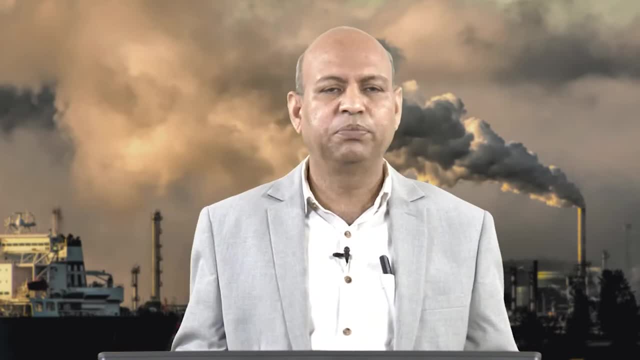 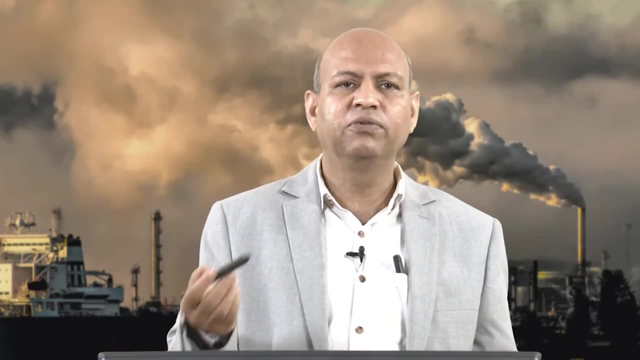 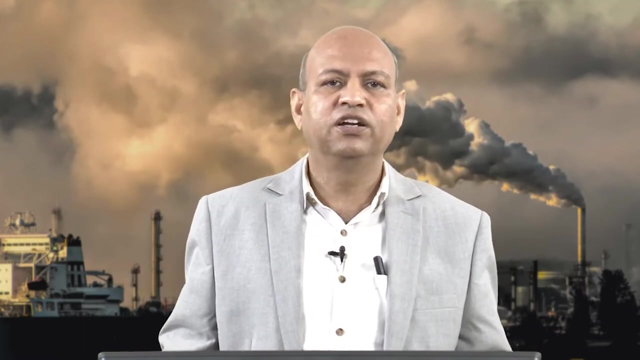 This is the type of fabric we should be using in that bag house filter. basically. Then, if you talk about like types of the fabric filters, then there are numerous types, like envelope type fabric filter can be there. It is in the form of cloth envelope supported on a wire screen frame and the individual 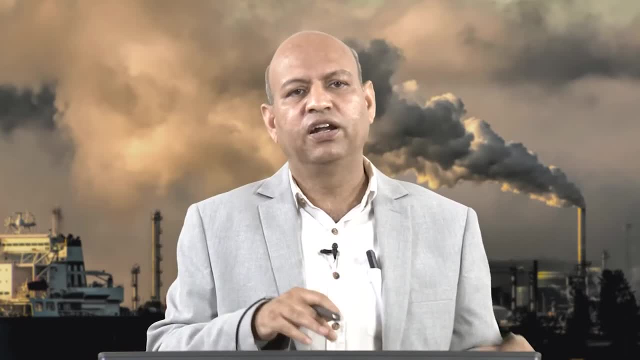 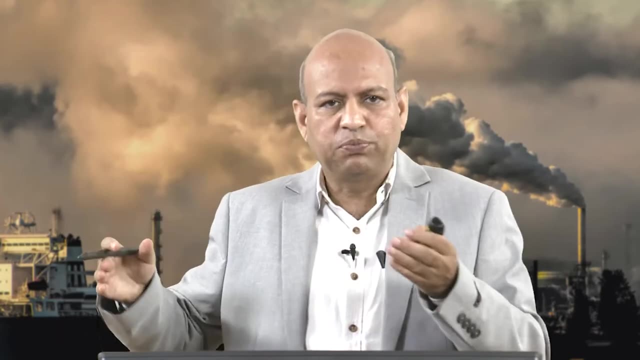 units range from around 0.6 to 1 meter wide and 3 to 5 centimeter thick, and gas is introduced on the outside of the each envelope. Okay, So it goes through the fabric into that frame of the unit and then it goes out of the collector. 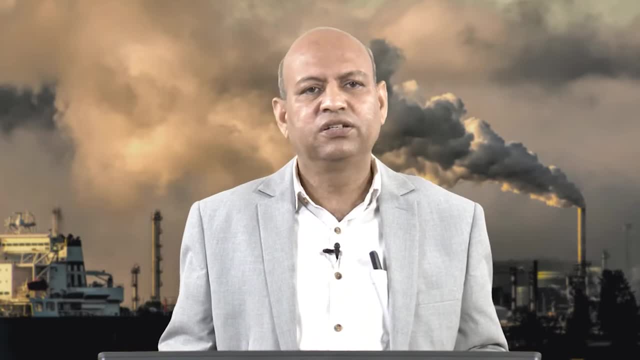 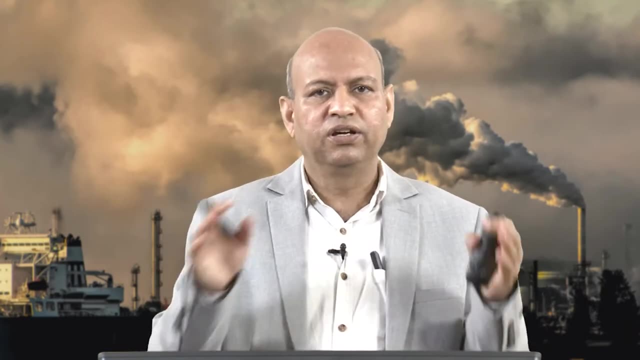 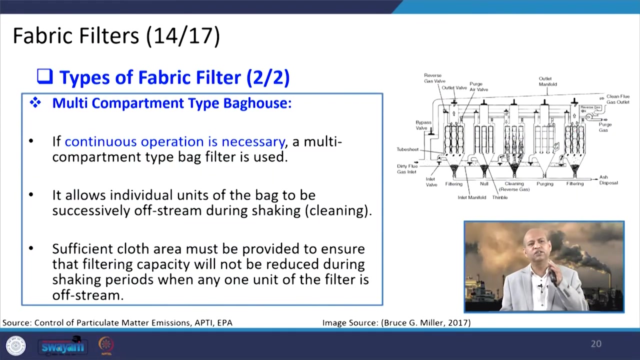 and then it, but it is not suitable for very fine particles, It is good for coarse particles, you can say. Then there may be multi compartment type bag house filters also, where different compartments are there, like 1,, 2,, 3,, 4,, 5, and for continuous operation is necessary. then these kinds of 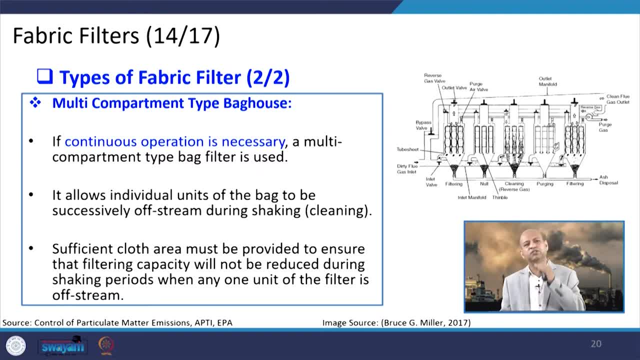 arrangements are very good because if one compartment is under maintenance then other compartments will continue to work. So those kinds of things can be there and then shaking, cleaning are needed for time to time. So some compartments will not be in operation but other compartments may be in the operation. 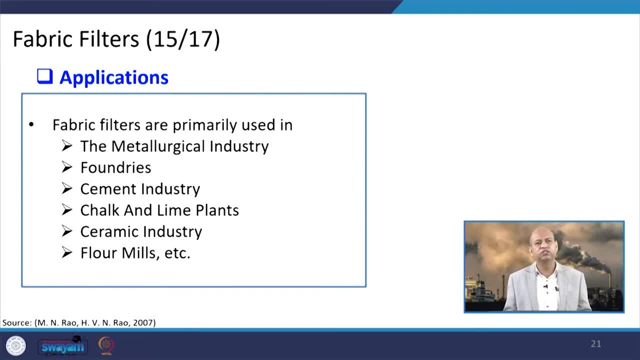 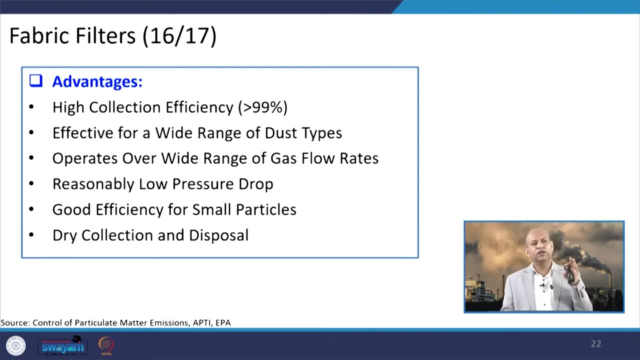 Then if we talk about like applications where they are good, these fabric filters, so we can see into metallurgical industries or foundries or cement industries, even chalk and lime plants, or ceramic industries, then floor mills, etc. So those are the kind of industries where these fabric filters are mostly used. 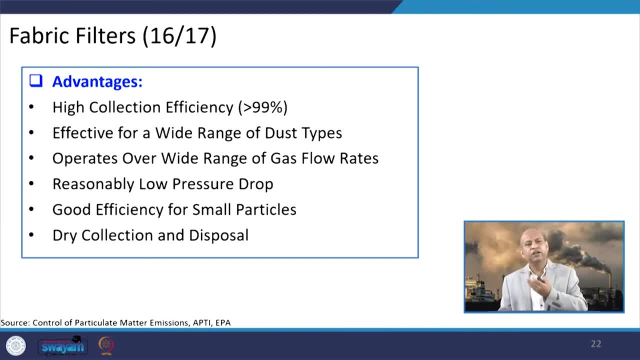 And the advantages if we talk about, then they are having high collection efficiency. even more than 99 percent of particles can be collected by fabric filters, And these are effective for a wide range of dust types, and this can operate over wide range of gas flow rates also. 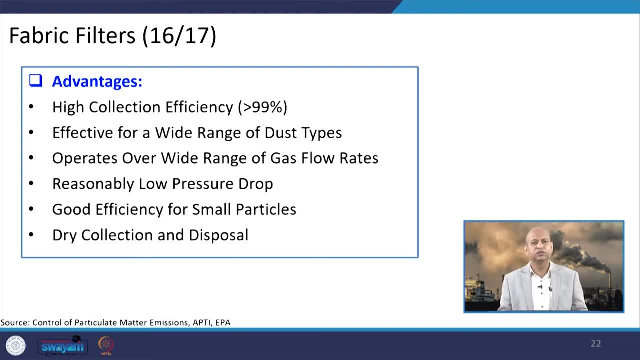 So fluctuation it can also afford to resist. Then reasonable low pressure drop is there. It is not very high pressure. High pressure drop, like other kind of devices, have good efficiency to small particles, also depending upon the pore size and then this flow rate etc. 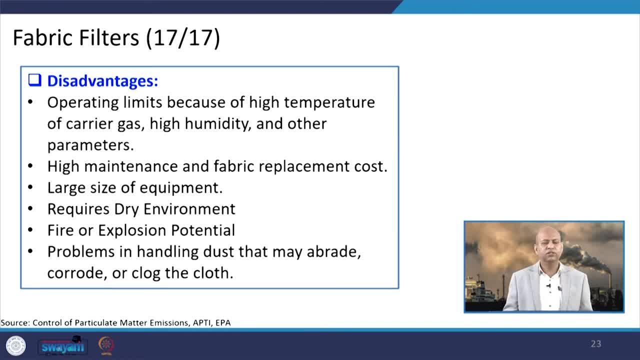 Dry collection and disposal is very good in that sense, but there are some disadvantages also, like there are limitations in terms of high temperature of carrier gas or high humidity and other parameters, because it cannot afford otherwise. very high temperature can generate some fire related problems. High humidity can very tight cakes may be formed and it is difficult to remove them. so efficiency decreases. High maintenance and fabric replacements cost can be there. large size of equipment is needed for, depending upon their flow rate. Then it requires dry environment. basically, moisture is not good for fabric filters And fire or explosion potential can be there, as I said, depending upon the temperature. 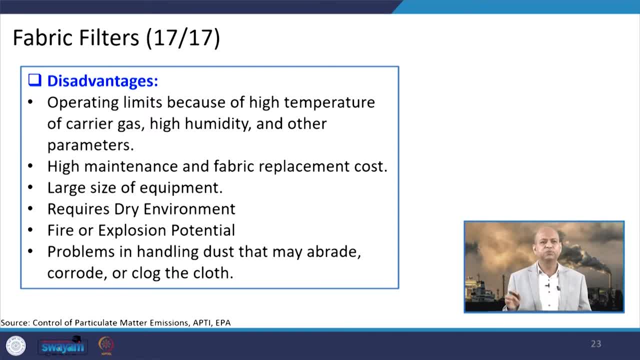 Problems in handling dust that may like corrosion. So these are the things: Corrosion kind of thing or clogging the cloth, so those kind of problems are there. it is not free from problems, But if we can get rid of these with highly skilled people and if you have lot of good. 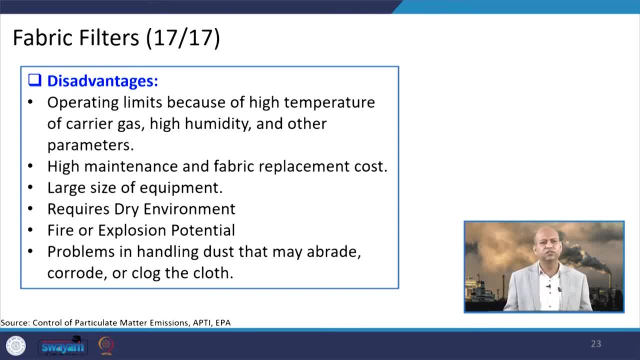 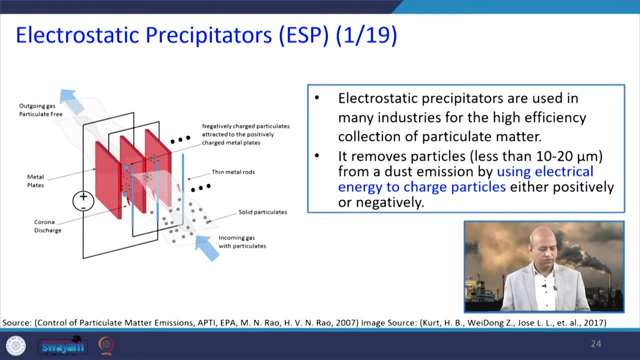 money to operate, then this is a good suggestion to go for fabric filter, depending upon if there is no very high hot gases there. Now, if we talk about electrostatic precipitators- Because fabric filters is Different device- electro precipitator is different device. 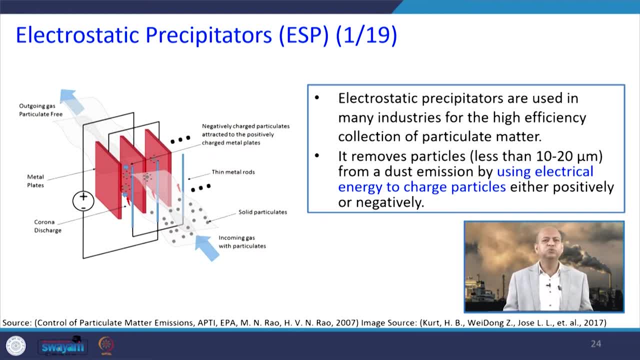 So if you talk about the electrostatic precipitators, they are used in mainly like industries of very high efficiency collection of particulate matter. We will see that they are very costly to install but their efficiency is very good. It can remove particles even less than point like less than 10 to 20 micrometer. 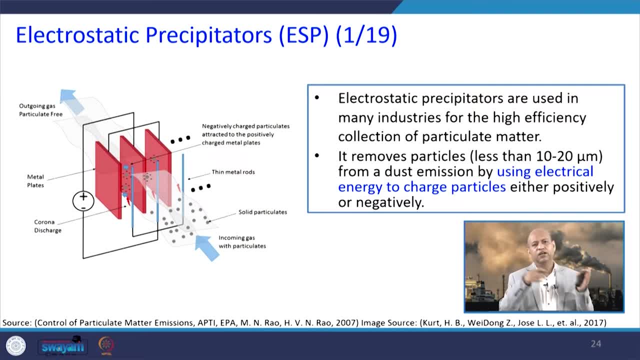 From a dust emission using electrical energy to charge particles and then go for the other kind of charge of the plates where they are deposited, because of opposite charge basically. So you can see here, one plate is there through which particles go through and they get charged. 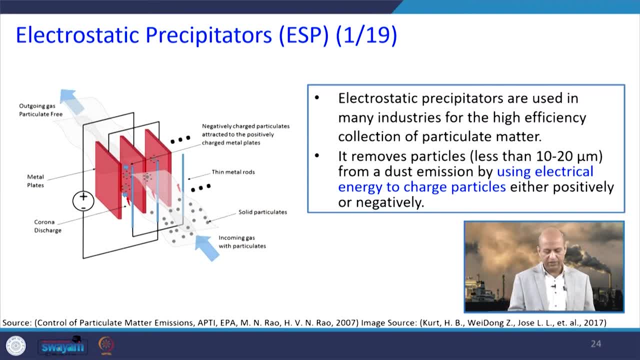 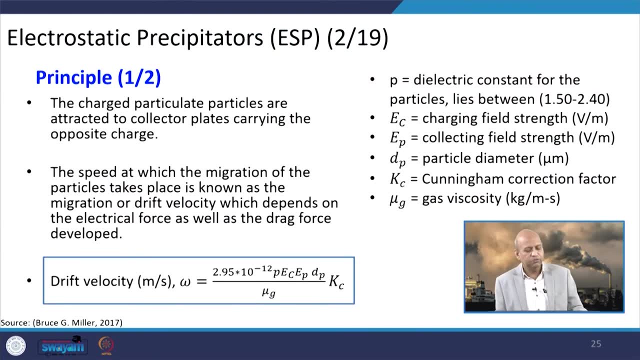 into that particular kind of electric charge and then they move towards the opposite charge plate where they lose their charge. So the charged particulate particles are attracted to the collector plates, basically carrying the opposite charge, And the speed at which they migrate from this charging plates to the collector plate can 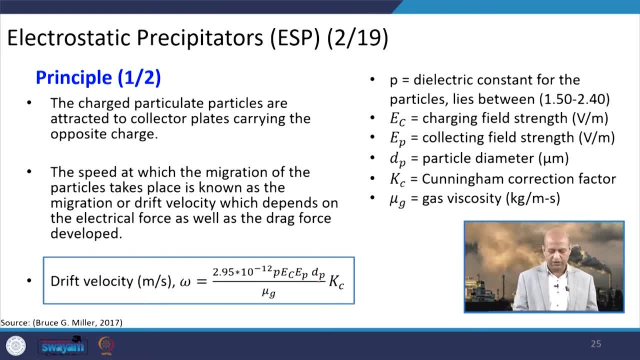 be known as the drift velocity, basically, And this can be calculated by this particular empirical relationship where we know, like this, dielectric constant for the particles which is between 1.5 to 2.4.. And then this EC charging field strength is there. 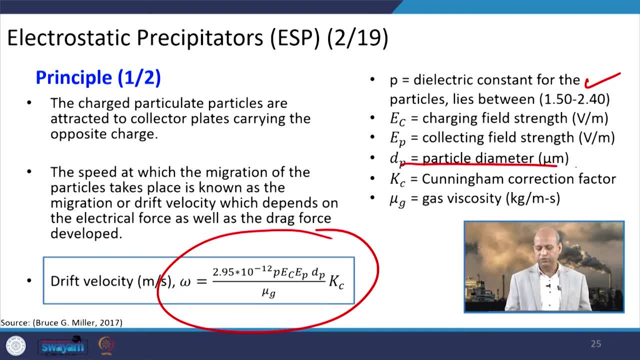 Okay, So dp collecting field strength, is there. dp is particle diameter- okay, this one. and the kc is correction factor. mu g is gas velocity. so all these sorry gas viscosity, so all these parameters are used for calculating the drift velocity. 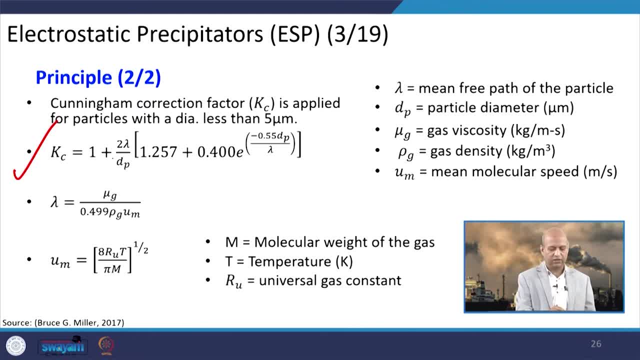 So these parameters, as we have seen, these are calculated by another set of empirical relationship where the meaning of different parameters are given. like free path of the particle mean free path particle diameter, So free path of the particle diameter. viscosity and gas density mean molecular speed, all. 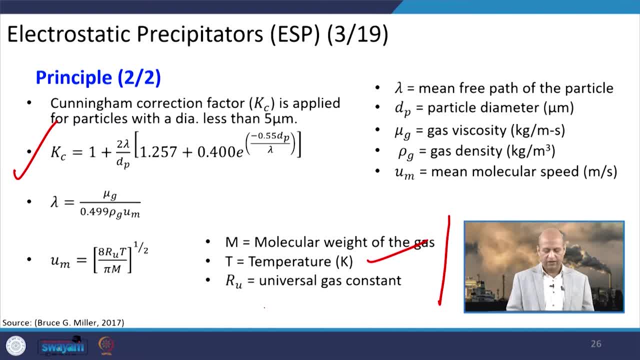 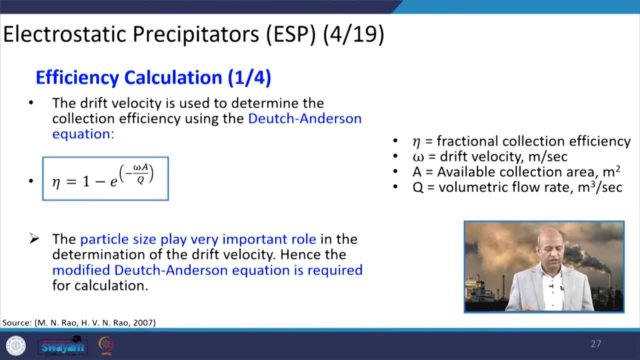 these, then molecular weight of the gas temperature in Kelvin and the universal gas constant is also used for calculation of this mu m. Then if we talk about efficiency of the collection, so that can be calculated by this formula, eta equals 1 minus e to the power of minus this omega a upon q. 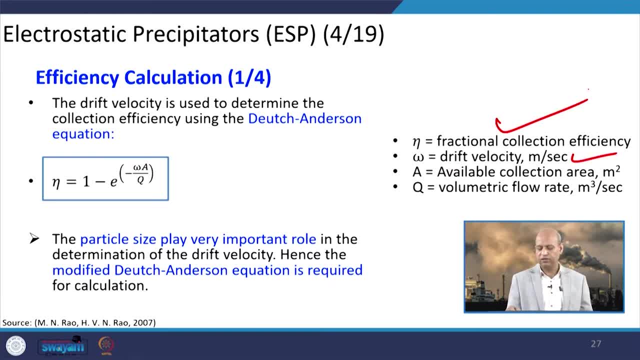 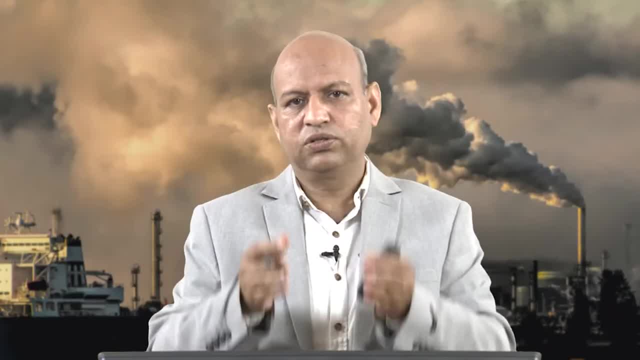 So you can see this omega s drift velocity, Okay, And eta is fractional collection efficiency. a is the available collection area of the plates. basically, if it is plate, if it is circular cylinder, then we can calculate the surface area, basically volumetric flow rate. q is there. 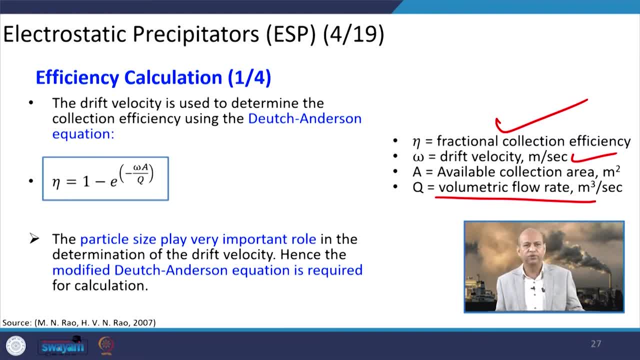 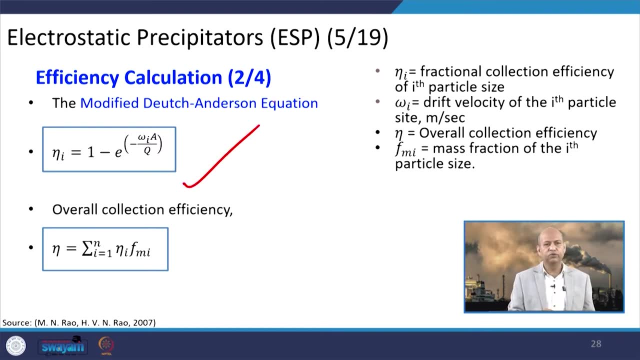 So the particle slice basically play very important role, you can see, in the determination of drift velocity, as we have seen earlier, and hence the modified this Deuce Anderson equation is required for calculations. Then this is the modified equation where you can use this wi- sorry, omega i. this is the 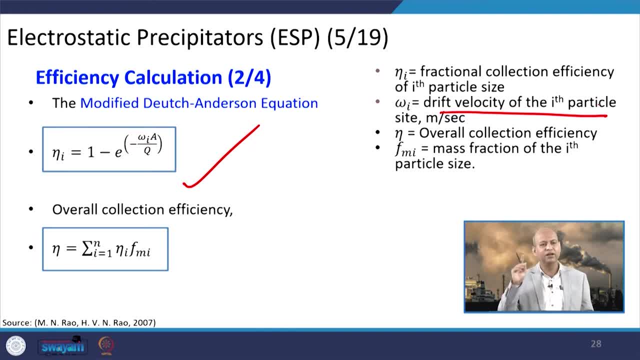 drift velocity of the ith particle. So different particle related calculations can be there and then we can do integration. So overall collection efficiency is there. this integration can be there for different type of particles and you can get the net collection efficiency Again if we see like efficiency. 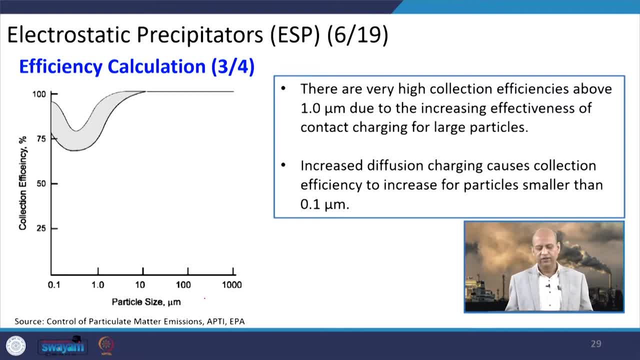 So different particle size collection efficiency is there and there are very high collection efficiency above 1 micrometer of the size of the particles when we talk about these electrostatic precipitators. but the increased diffusion charging causes collection efficiency to increase for particles smaller than even 0.1 micrometer. 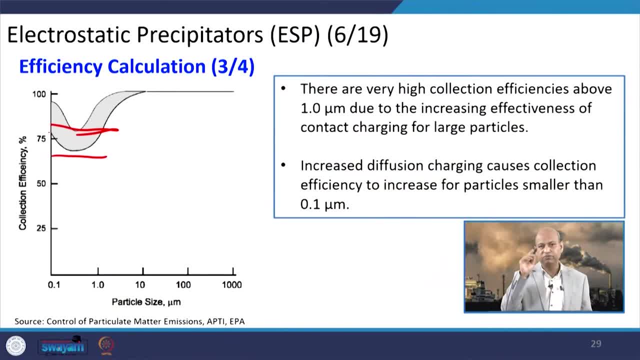 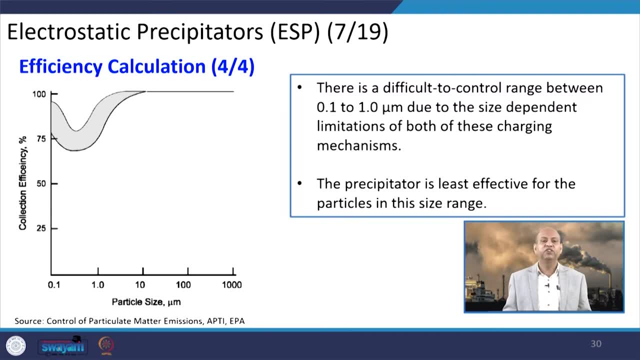 So that kind of efficiency also increases here, as we have seen in the back filter or fabric filter kind of devices. Okay, Well, there is a difficult to control range between this 0.1 to 1 micrometer due to the size dependent limitations. 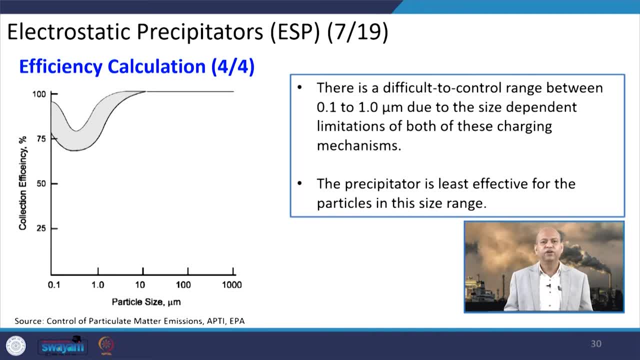 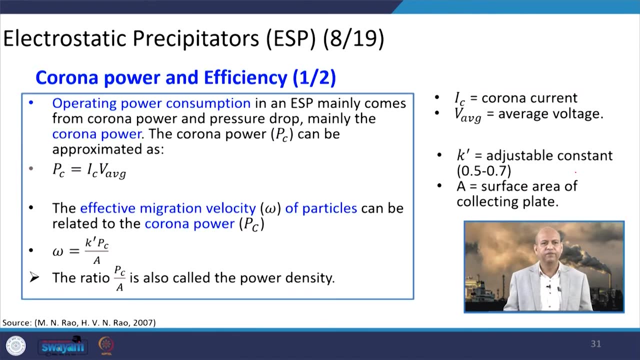 So these precipitators are least effective when for this particular size range. but, as we have seen, little bit improvement can be there depending upon this diffusion, charging kind of phenomena. Okay When we talk about like. Okay When we talk about like corona power and efficiency. so you see, this is operating power consumption. 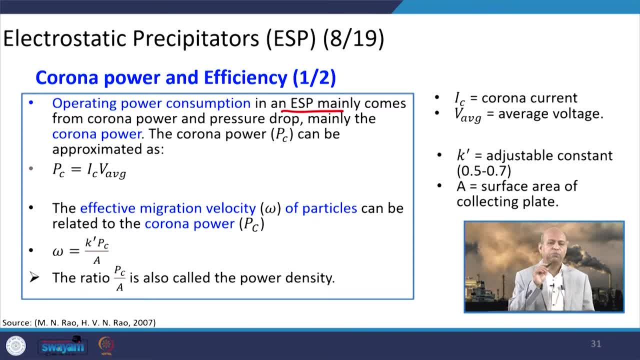 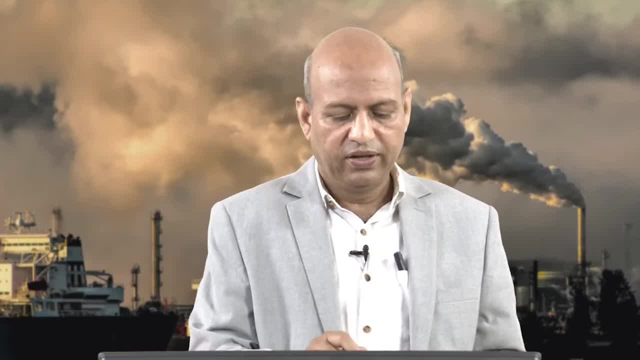 in electrostatic precipitator which comes from the corona power. where this some blue light is there, where this passes through, gas and particles pass through, we call it corona. So this corona power can be calculated by this particular relationship where IC is corona. 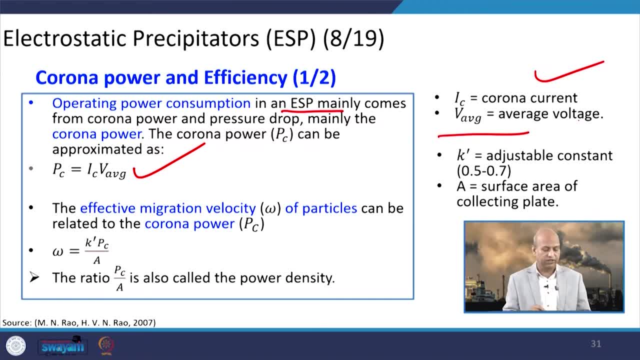 current and this VA average is average voltage basically Okay. So this adjustable constant is there, surface area of the collecting plate is there. so you can calculate this omega K dash PC divided by A, and this ratio, PC by A, is called power. 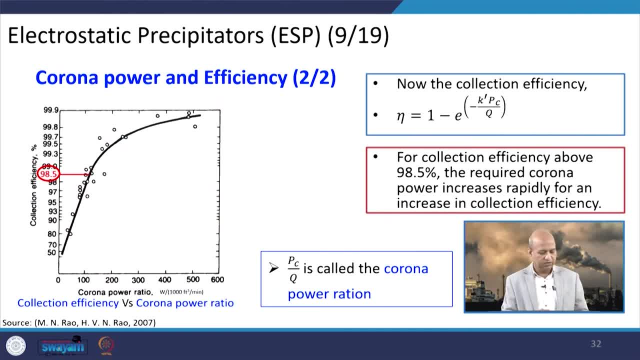 density here in this particular relationship. When we see this corona power ratio and collection efficiency, you can see there is one good range where 98.5 percent efficiency can be achieved. Okay, So with this relationship we can calculate this net collection efficiency. and as it is, 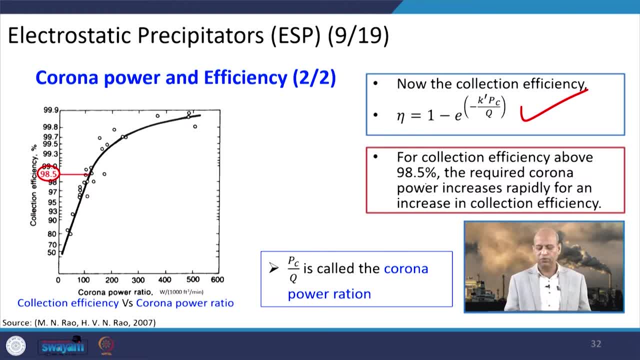 given in this particular figure that the collection efficiency above 98.5 percent. this required corona power increases rapidly for an increase in collection efficiency. So up to this it goes very rapidly, but after that it is slightly slow. you can say: 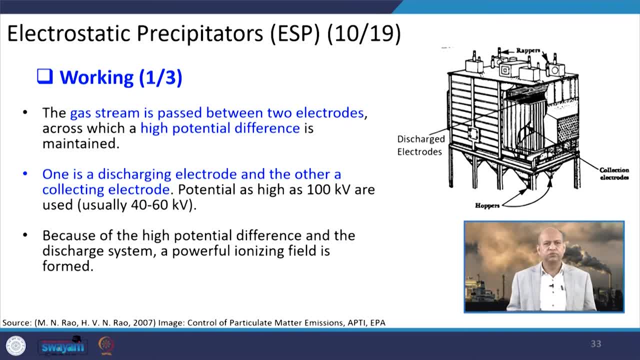 So, if you talk about like working, how does it work basically? So the gas stream is passed between two electrodes across with a high potential. difference is maintained between those two electrodes: one is a discharging electrode and the other is collecting electrode, where these particles go and lose their charges. 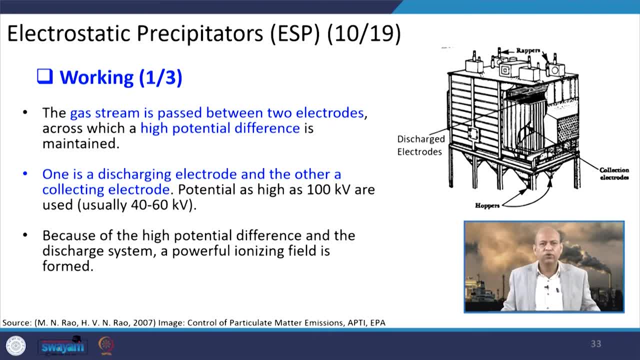 And the potential as high as 100 kilo volt are used. usually 40 to 60 kilo volt is the voltage there, but 100 can also be there. because of the high potential difference and the discharge system, a powerful ionizing field is formed where these particles get ionized. basically. 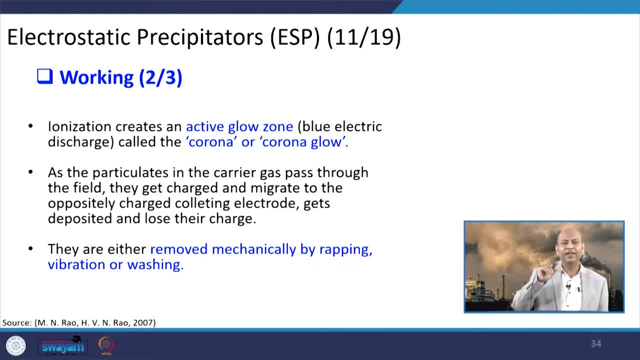 So ionization creates an active glow zone like blue electric discharge, you can say that is why we call it discharging zone and this is called the corona or corona glow, So as the particulate matter pass through this carrier gas with the particles, when 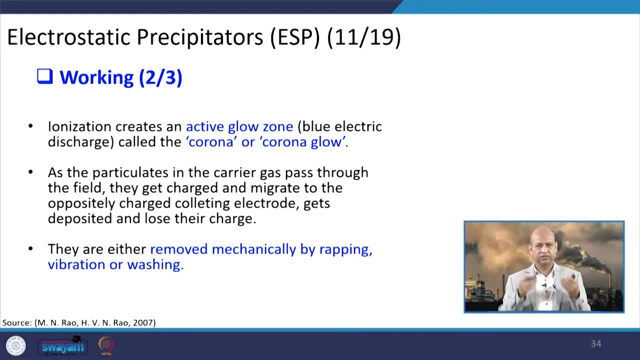 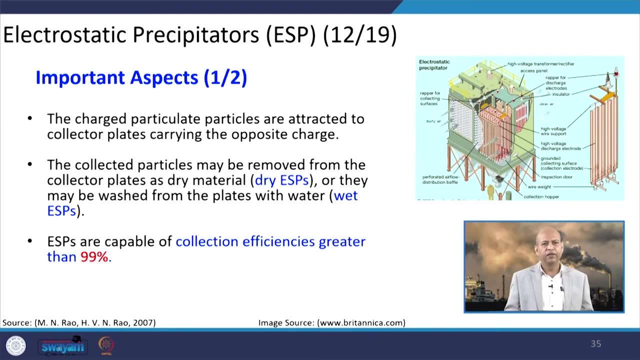 it pass through this particular field, they get charged. These particles get charged and then it goes to the collecting electrode where they lose the charge basically and slide down to the bottom where hopper is there and it is removed periodically. There are some important aspects. for example, the charged particles are attracted to collector. 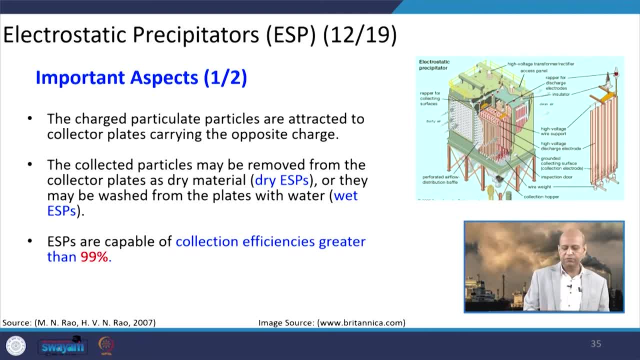 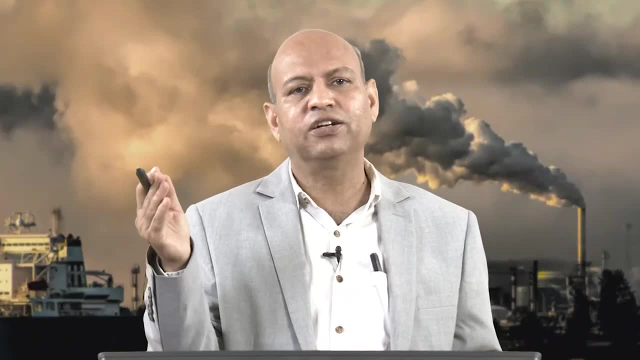 plates carrying the opposite charge. The collected particles may be removed from the collector plates and this dry material, that is, a dry ESPs, Or they may be washed from the plates with water wet ESPs. so two kinds of ESPs may be there: dry electrostatic precipitators or wet electrostatic precipitator, depending. 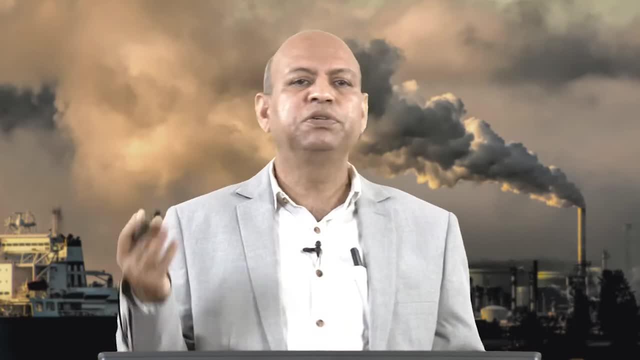 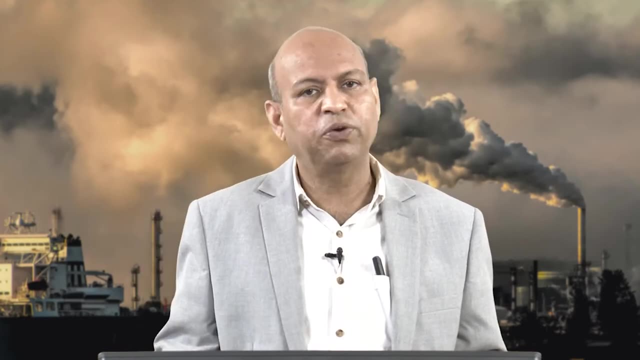 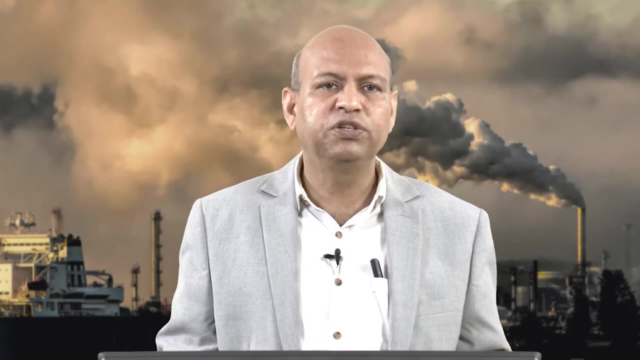 upon. how do we remove the particles. So these ESPs are capable of correction efficiencies greater than 99 percent, even 99.9 percent sometimes. those kinds of efficiency can be achieved by electrostatic precipitators, And the design parameters which affect the efficiency of ESP are like volumetric flow. 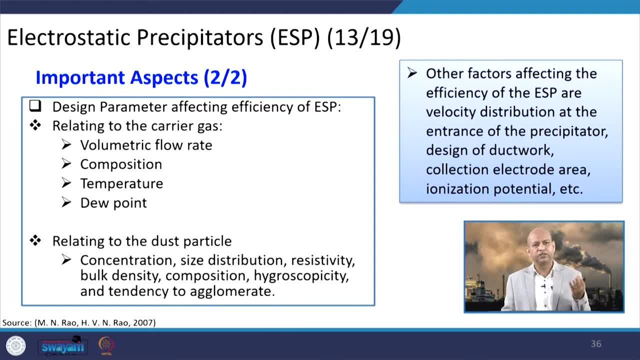 rate, composition of the gas and particles, temperature, dew point. if dew point is there, then some acidic formation is there that they can attack the plates, etc. Then there are like relating to the dust particles, for example concentration or size, distribution of the particles, resistivity, then the bulk density and composition, or hygrospic nature. 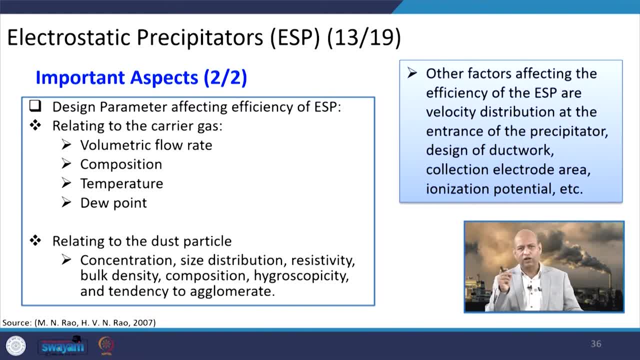 like moisture can be contained or tendency to agglomeration. those kinds of things are there. So the factors affecting the efficiency of ESP are like velocity distribution at the entrance of this precipitator, then design of this dock work and collection electrode. 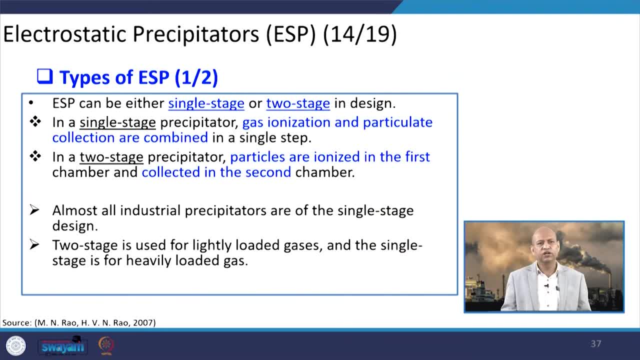 areas and ionization related potential. those kinds of issues can be there which are important when we do design of the electrostatic precipitators, And these can be either single stage type or two stage type. basically, In a single stage type precipitator, this gas, ionization of the particulate matter and 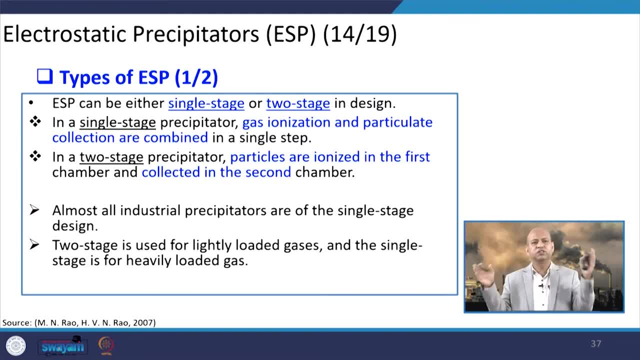 collection are combining with single step within the single chamber. you can say At one corner it goes, another corner they get collected and goes down In two stage. one chamber is for like this kind of ionization of the particles, other is for this collection or deposition of the particles. 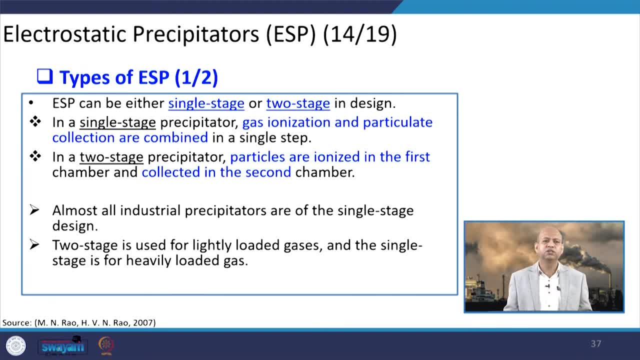 And almost all industrial precipitators are of the single stage design. basically two stage is used for, like, lightly loaded gases. So these are the two stages- Lightly loaded gases and the single stage is for heavily loaded gases. So those are the basically differences. 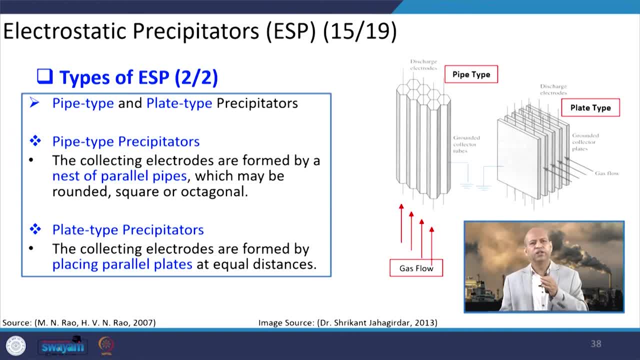 Then different types are, also in terms of their shape, like pipe types can be there. these kind of formation may be there: different pipes. gas passes through these pipes and then up to their wall. they trap and then go down. Then these may be plates type, so different kind of shape may be there. 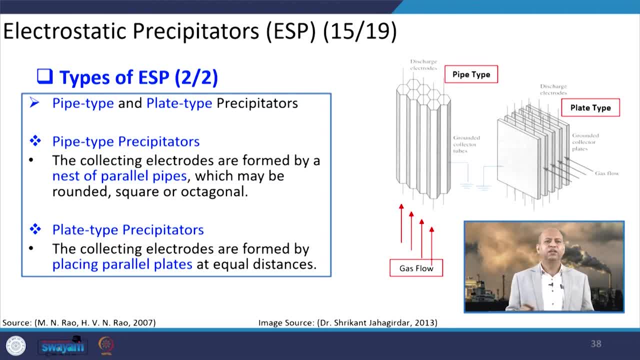 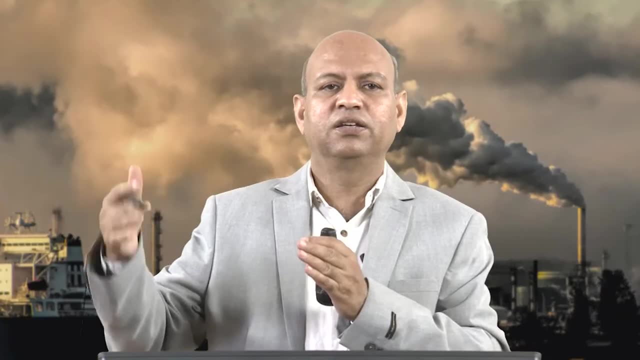 So the collecting electrodes are formed by a nest In parallel pipes in the pipe type precipitators which may be rounded or square or octagonal in shape, basically, So there may be long pipes of different shapes. Plate type are like, they are in parallel. they are parallel plates which are at equal 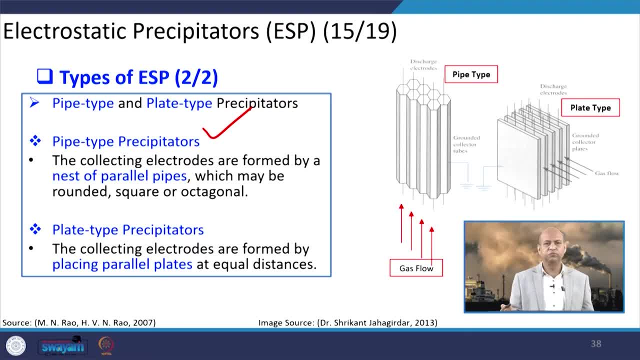 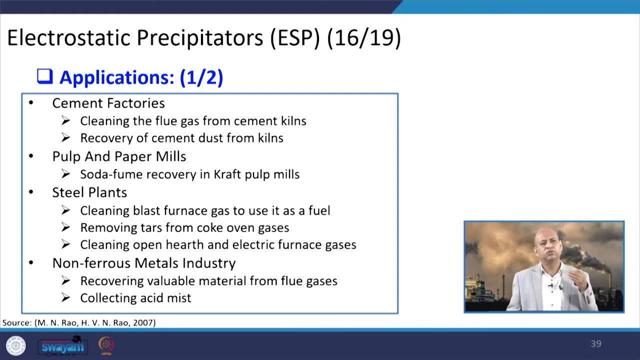 distances. they are kept and accordingly, the gas laden with particles are passed through those openings. Well, when we talk about application, so they are very popular in industries like cement factories. So cleaning the flue gas from cement kilns or recovery of the cement dust from the kilns. 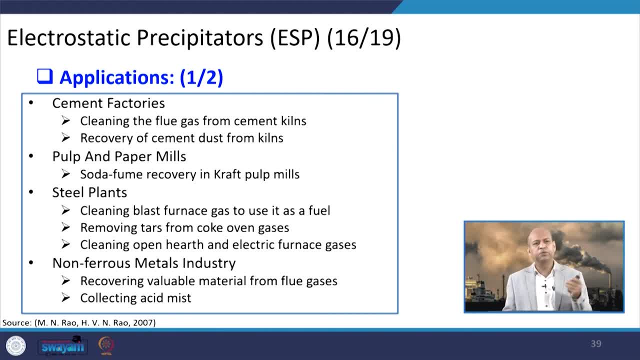 those kind of things can be done by these ESPs: Pulp and paper mills or soda fume recovery in craft pulp mills. again, ESPs are very good Steel plants where cleaning blast furnace gas to use it as a fuel. So fuel recovery is done by ESPs. 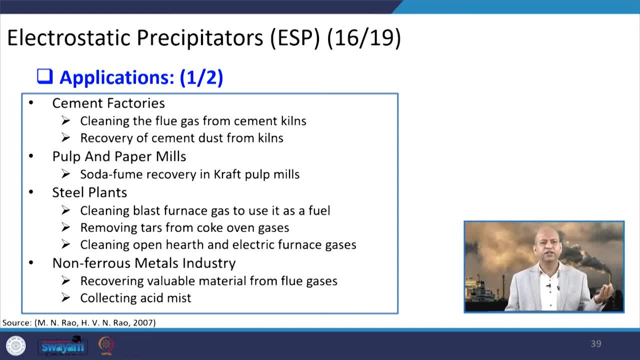 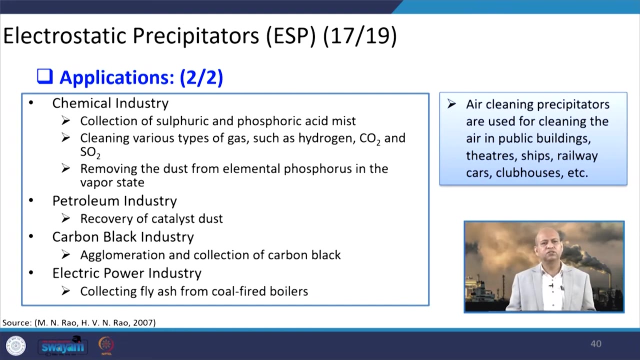 Removing these tars from coke over gases or clay, These cleaning open hearth and electric furnace gases. that can be done by ESPs. also. Non-ferrous and metal industries also use in a significant manner or large manner these ESPs: Chemical industries, petroleum industries, carbon black industry or electric power industries. 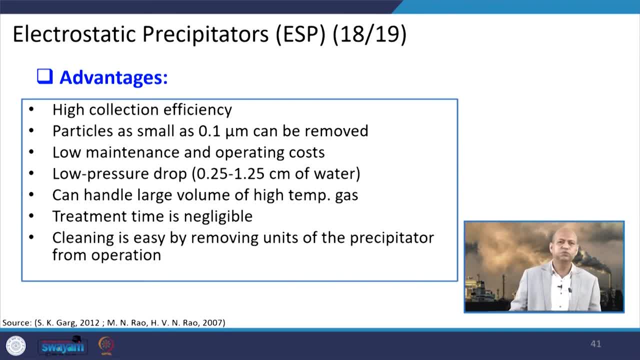 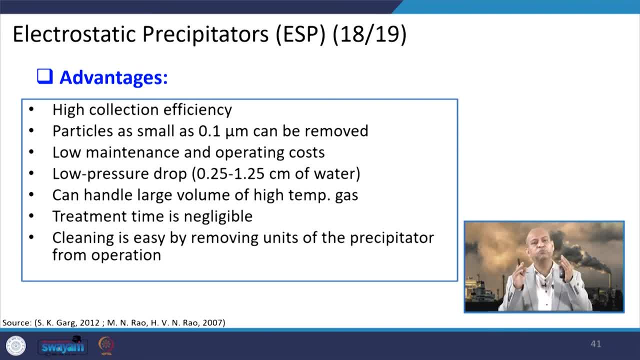 So these ESPs are very popular. So these ESPs are very popular, So the big advantage of these ESPs- and, as I said, even 0.1 micrometer can be removed, So this is great range in that sense. 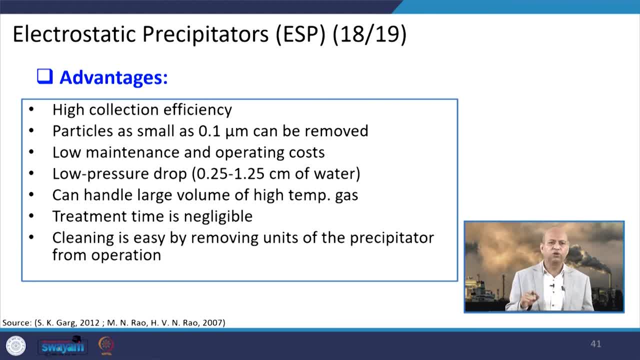 Low maintenance and operating cost or low pressure drop and then it can be handling large volumes of the gases. basically, even up to high temperature treatment time is negligible- very quickly. it removes. basically Cleaning is easy by removing units of the precipitator from operation, but there are. 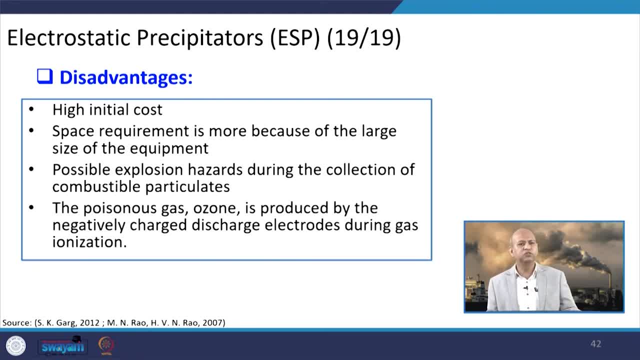 disadvantages or limitations. But there are disadvantages or limitations. initial cost is very high. So those industries which do not have good funds for that, they cannot afford this kind of device. Space requirement is also more because of the large size of the equipment and the possible explosion hazard can be there. collection of combustible. 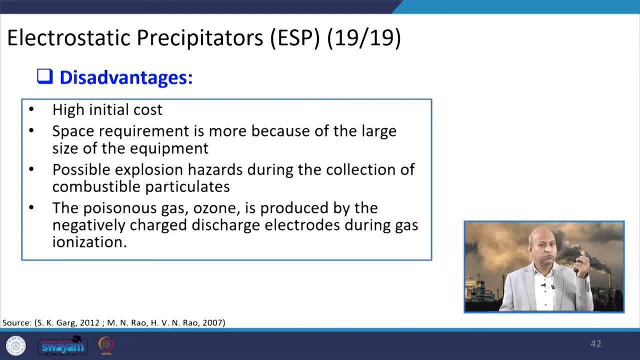 particulates can be there because of this ionization, and sometimes ozone is formed in that. So this kind of problems may be there. Poisonous gas, ozone, is produced by the negatively charged discharge electrodes during the gas ionization, So very skilled person must be there. 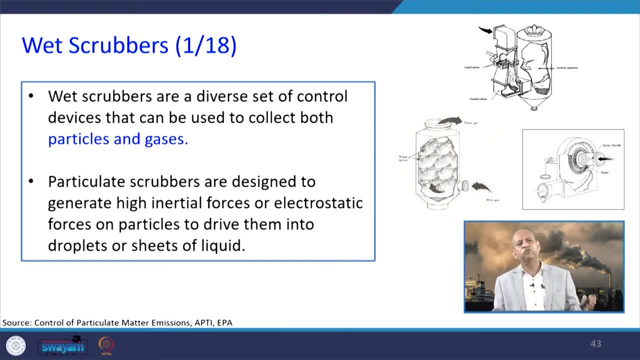 to handle it or to operate it. Now we talk about the wet scrubbers. This is third kind of device in today's lecture. basically. So these are the devices or scrubbers, which are diverse set of control devices which can be used for collecting both particulate matters as well as. 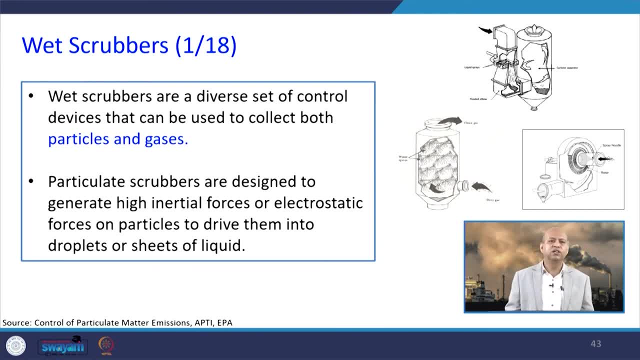 gases. So particulate scrubbers are designed to generate high inertial energy. So particulate scrubbers are designed to generate high inertial energy, So they are designed for controlling the forces or electrostatic forces or particles to drive them into some kind of droplets or sheets of the liquid where liquid is. 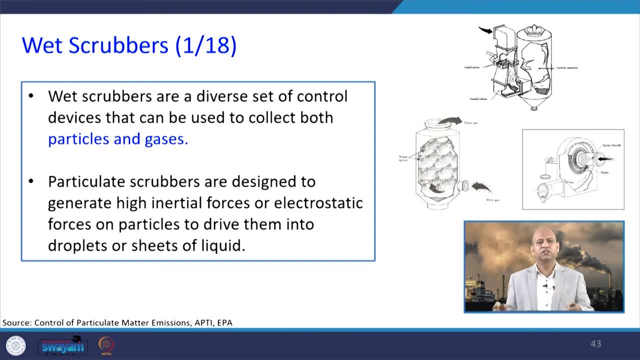 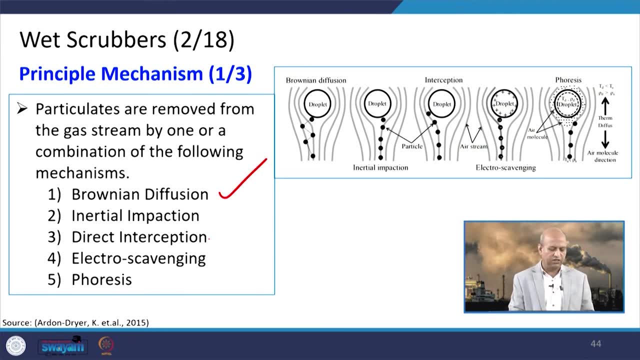 dropping in a kind of sheet So they can get attached to this and removed, And the principle. if you talk, then there are the certain mechanism like Brownian diffusion, inertial impacts and direct interception, electro scavenging and phoresis. all these kind of mechanism can be used for 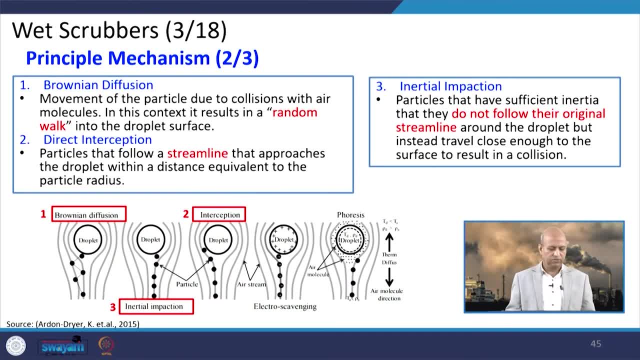 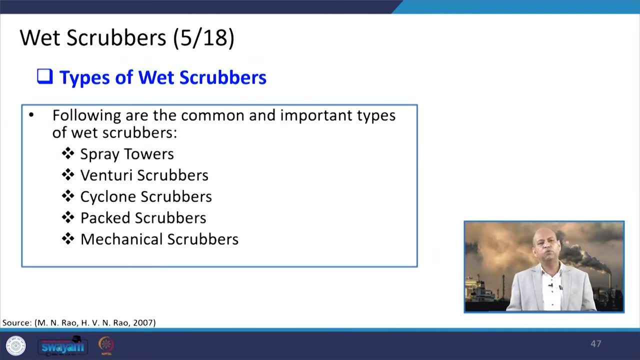 wet scrubbers basically. So these are like random, which we have seen in earlier, also Brownian diffusion, direct interception, depending upon where you are targeting that particular stream. So these kind of mechanisms are used very frequently. If you talk about different types of wet scrubbers, then there can be like spray towers or wanchery. 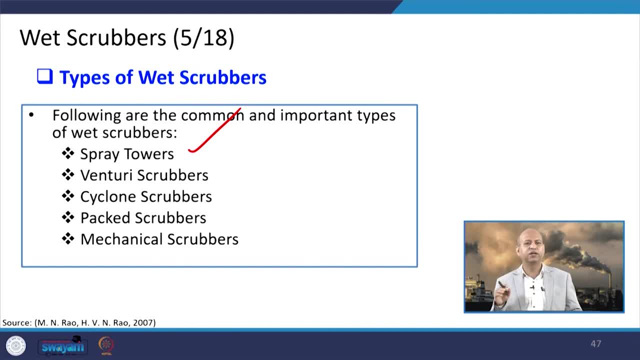 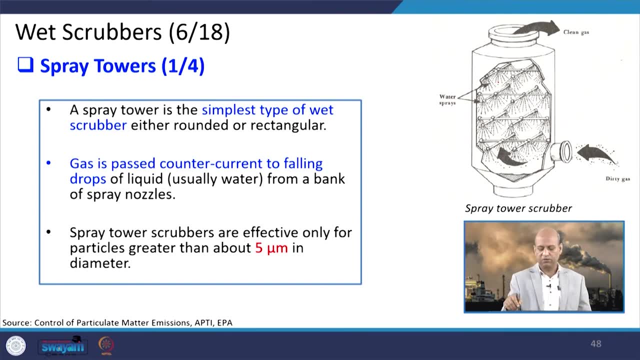 scrubbers or cyclone scrubbers or packed scrubbers or mechanical scrubbers. So if you go one by one in a spray towers, you can see this kind of tower is there and spray means some water spray can be there or some solution can be sprayed, depending 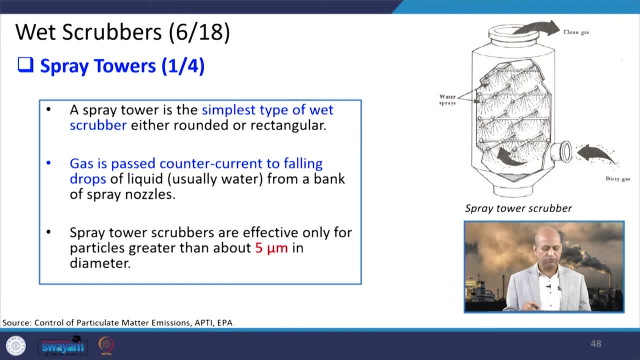 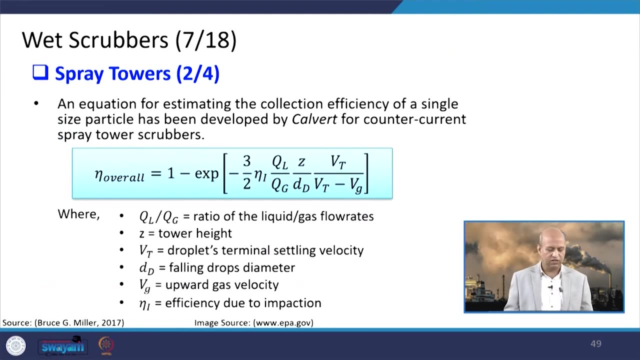 upon, what kind of gases are there, what kind of removal efficiency is needed. So this is the device which is known as a spray tower scrubber, and it can effectively remove particles even greater than 5 micrometer in size. up to 5 micrometer size, it can remove. 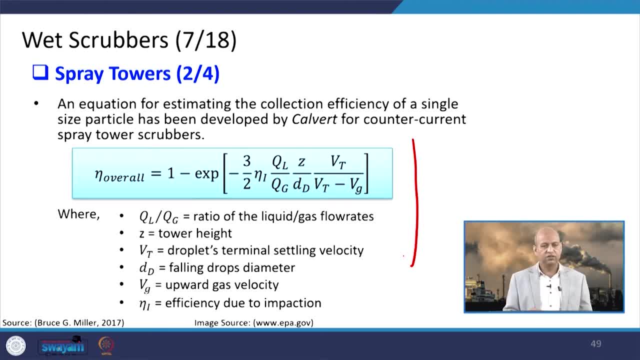 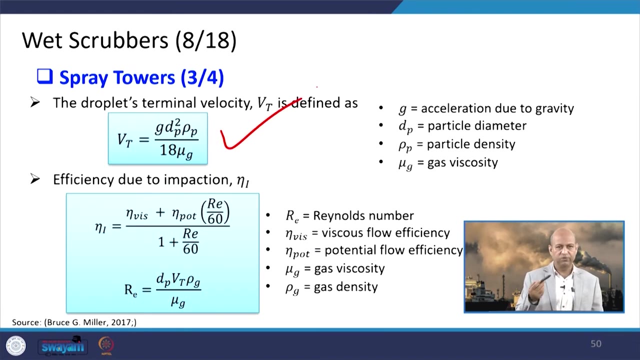 This is the overall, So this is the efficiency which is calculated. this relationship for spray towers, where these tower height z, and then droplets terminal settling velocity, then falling drops diameter and the upward gas velocity, efficiency due to impaction. all these parameters are used on right side in the empirical relationship. then terminal velocity: how to calculate earlier. 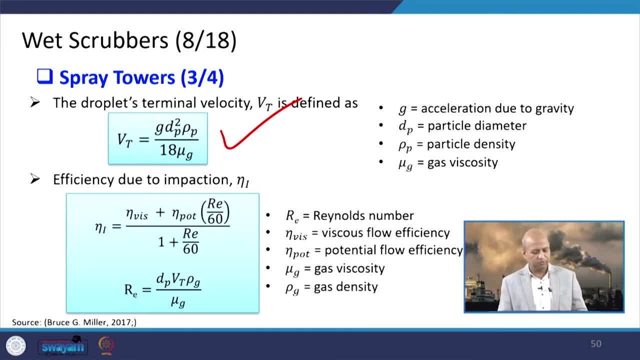 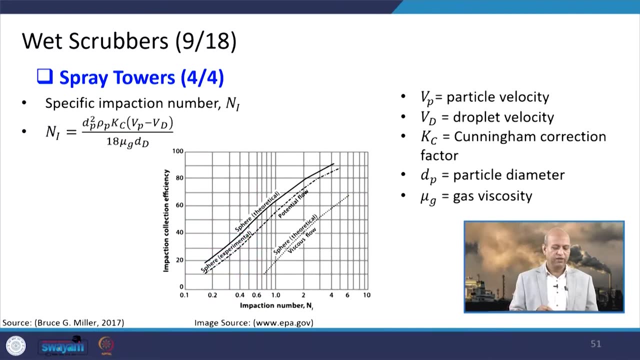 we have seen in case of that settling chamber also, And this efficiency of impaction. However, impaction can be calculated by Reynolds number. viscous flow efficiency, potential flow efficiency, gas viscosity, gas density- all these kind of parameters are used in these empirical relationship And then specific impaction number is calculated by these kind of relationship or graphs or 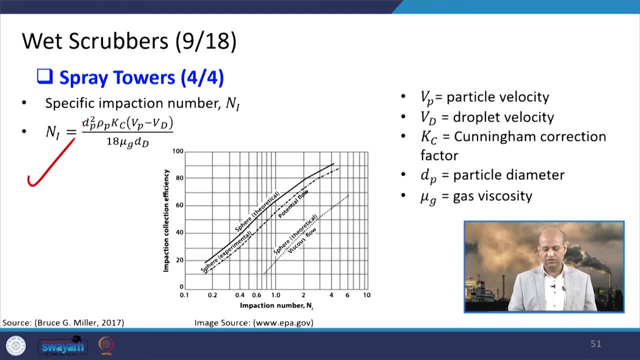 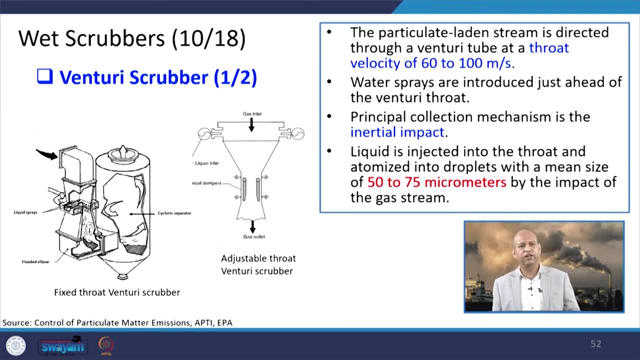 charts. So you put those values and you can get this n1. that is the specific impaction number. when we talk about different scrubber, like wanchery scrubber, Then there there, we use very narrow throat to push liquid these particles with high speed and at the 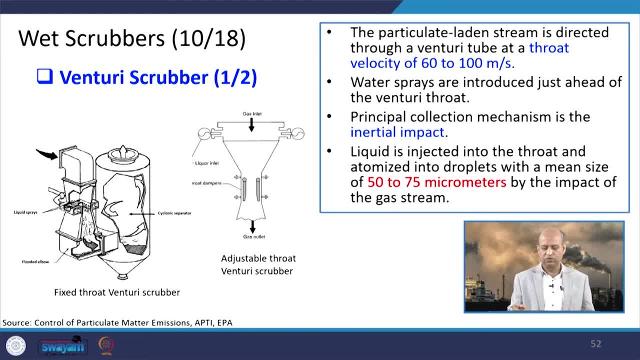 same time liquid also after certain distance. So this velocity like 60 to 100 meter per second, very high velocity through the throat, and water sprays are introduced just ahead of the venturi throat So this inertial impaction is occurred and that can remove these particles and this mean 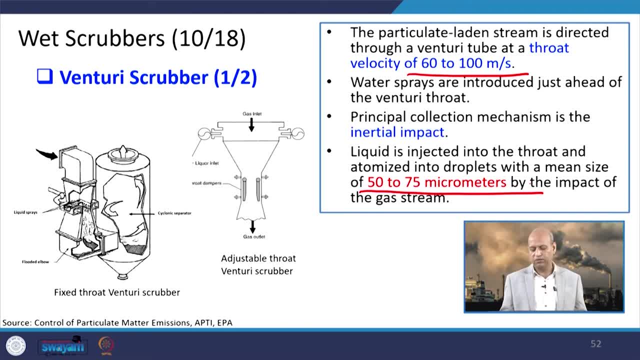 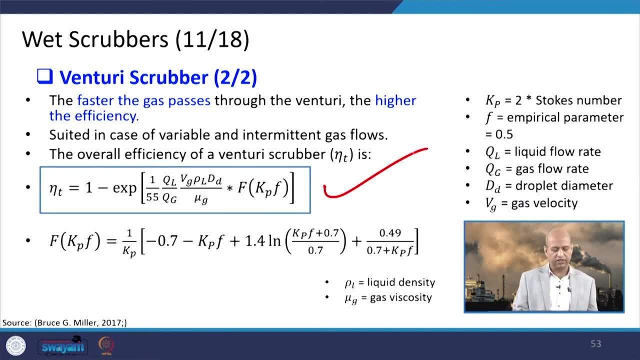 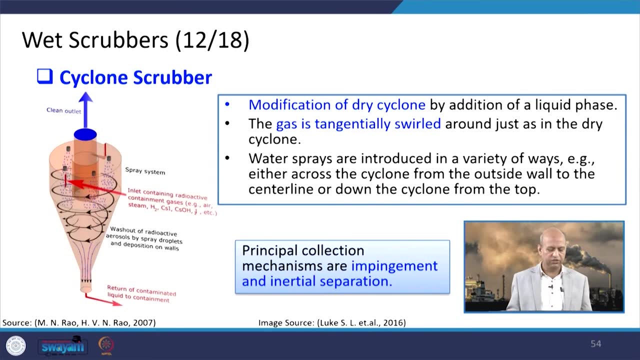 size like 50 to 75 micrometer particle of the size particles can get removed very easily. These are the empirical relationships for calculation of efficiencies. again, these liquid density, gas viscosity, all those parameters are used basically When we talk about cyclone scrubbers. then there is modification like we have seen dry. 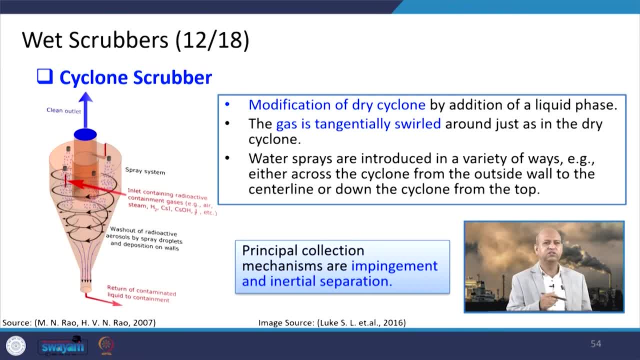 cyclones for particulate matter. In this some liquid is also used, Also spray sprayed. You can see that can be this. water spray can be in this tube when gas goes up, or it can be at the side, also depending upon which kind of design you are taking into account. 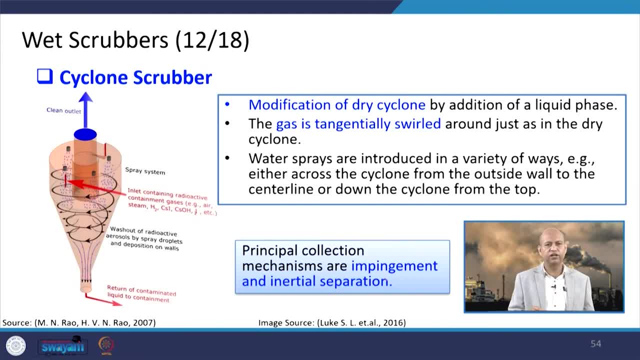 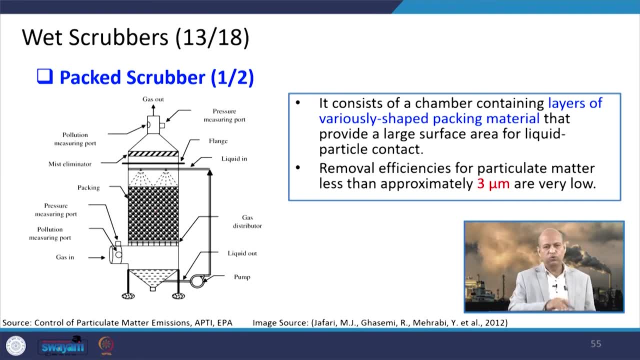 So for impingement and the inertial separation. these kind of mechanism are used with cyclone scrubbers. Packed scrubbers are using some sort of materials to provide large surface area where the particles can get attached, As well as sprays. 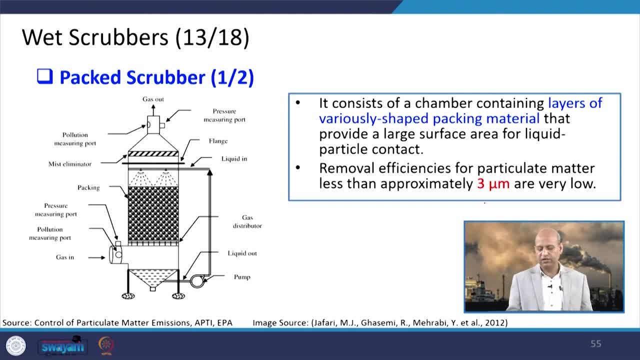 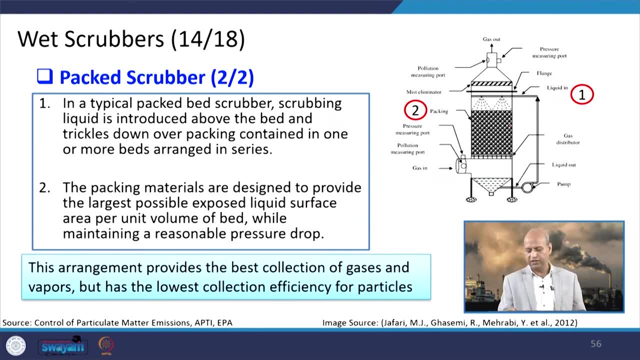 So also there of the sub solution. So the packed material must be there and it can remove up to 3 micrometer of the particles, And you can see this packing material here and liquid is taken into like a spray. So this arrangement provides the best collection of gases and vapors and lowest collection. 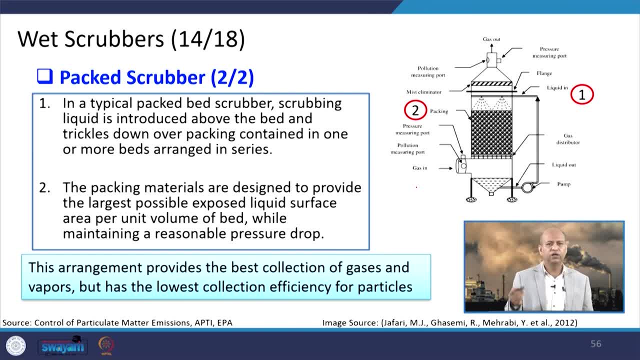 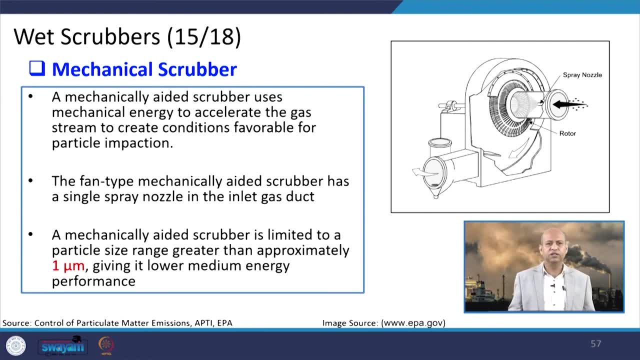 efficiency for particles basically. So they are more into removal of the gaseous emissions. basically, When we talk about mechanical scrubbers, So this is the mechanical scrubbers, So these are mechanically aided scrubber. basically, You can see here a spray nozzle can be there and this fan type mechanically aided scrubber. 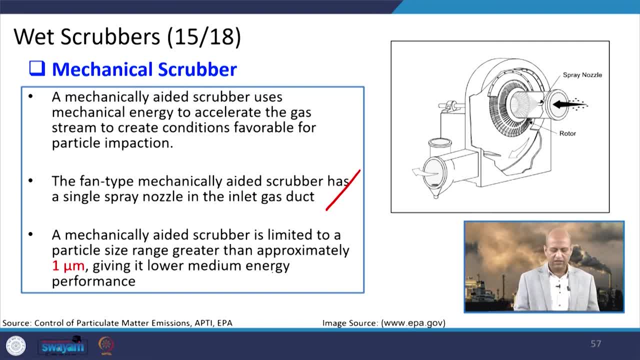 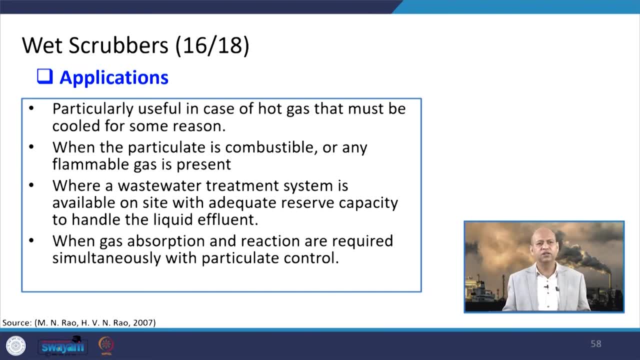 can be there, So efficiency is increased in that sense, and it can go up to 1 micrometer size to remove the particles. Well, applications of wet scrubbers are like. it is useful for both gas as well as particulate removal, And it must be cooled for some reason. 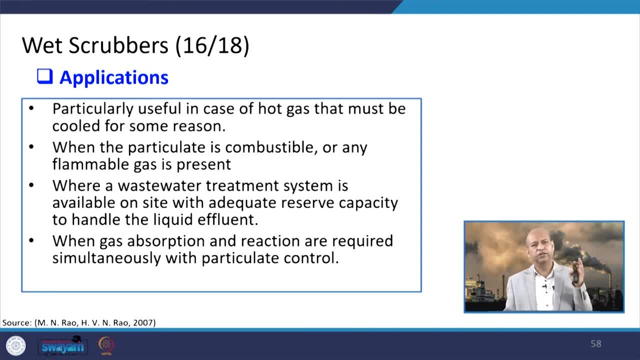 So then scrubber can be removed. Wet scrubbers are needed, not other kind of devices. So that way scrubbers are good for that purpose, where hot gases are there and we need to dampen its temperature before removal of other particulate matter or gases. 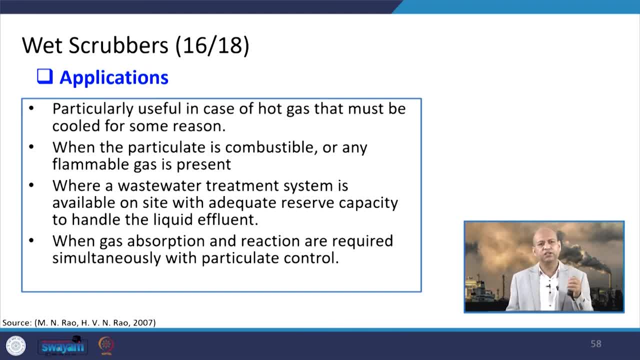 When the particulate is combustible or any flammable gas is present, then also wet scrubbers are better because they will not have this fire related problems Where a waste water treatment system is available on site with adequate reserve capacity to handle the energy. 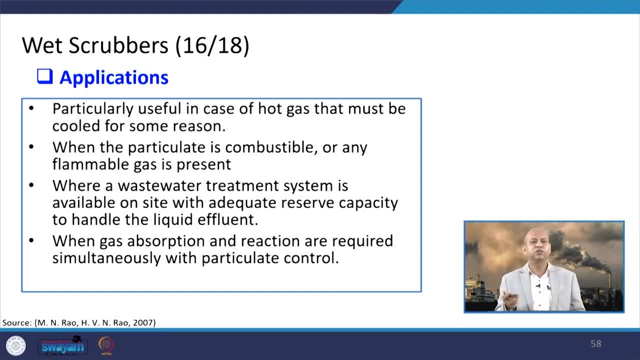 So there is no liquid effluent. Otherwise we will have to have this waste water treatment plant because wet scrubbers are producing waste water basically. So air pollution is converted into waste water. you can say in that sense When gas absorption and reactions are required simultaneously with particulate control. 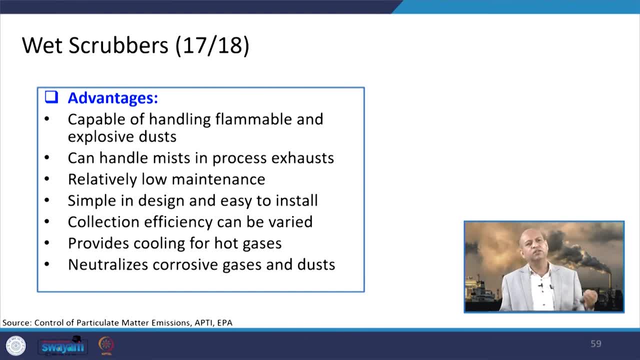 So those where applications are more popular. Then there are advantages, like it can be capable for handling flammable and explosive dusts, because wet scrubber is there, water and those kind of things. It can handle mist and in the process of exhaust. then relatively low maintenance is required. 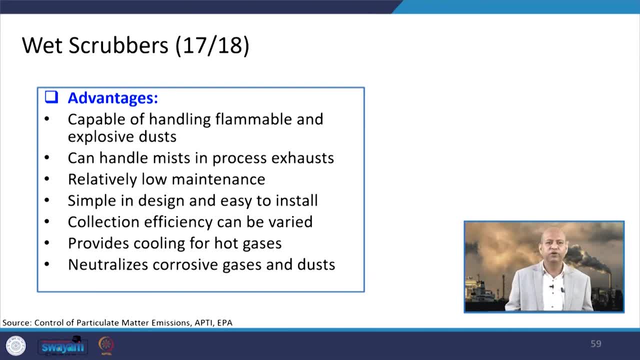 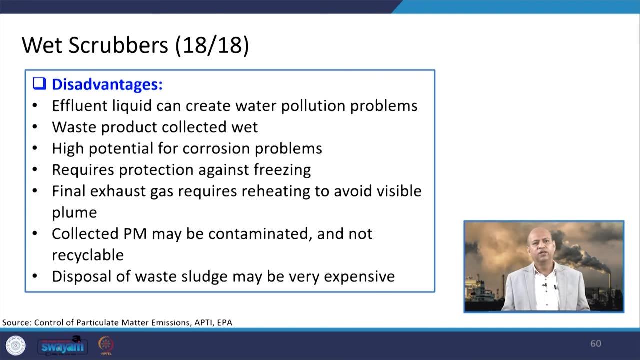 simple in design and easy to install. collection efficiency can be varied depending upon different size and nature of the particles. provides cooling for hot gases, so neutralizes corrosive gases and dusts. So those kind of advantages are there, but of course limitations are also there, like 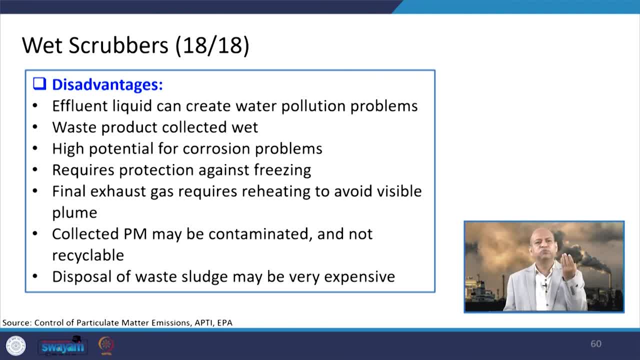 effluent liquid can be in the form of some water pollution. So another problem has been created So we have to deal with it. Waste product collected like in wet position, not dry, So handling is difficult. Dry it is very easy to handle. you can just go and dump it somewhere or you can use in. 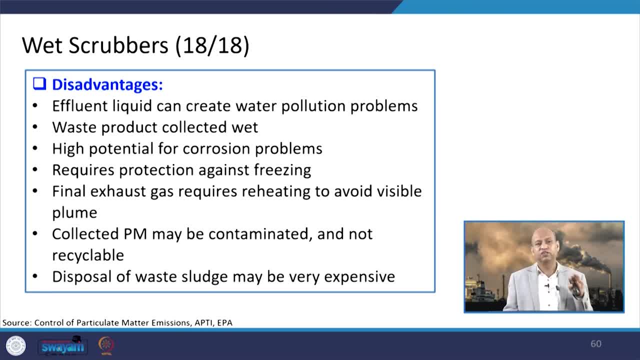 some other form. High potential for corrosion problems can be there because this moisture and if acidic gases are there, It requires protection against freezing. So it is very easy to handle If it is freezing because water is there. so in very cold regions it is difficult to. 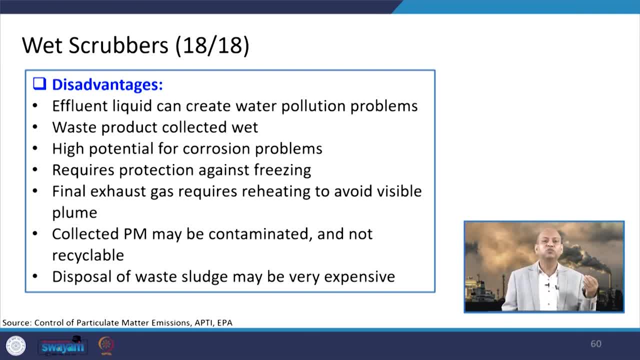 run. Final exhaust gas requires reheating to avoid visible plumes. otherwise, even if water vapor is coming out, people think it is a lot of pollution. perception can be there. Collected particulate matter may be contaminated and not recyclable. as I said, dry could be.